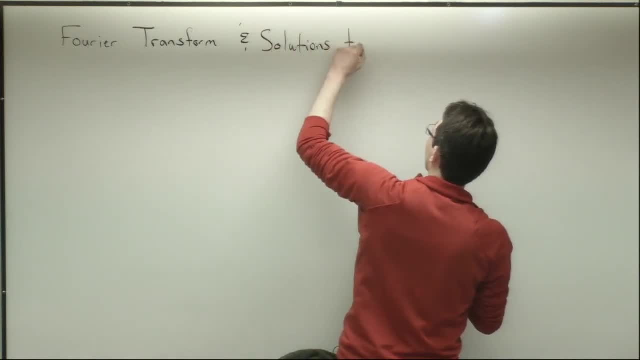 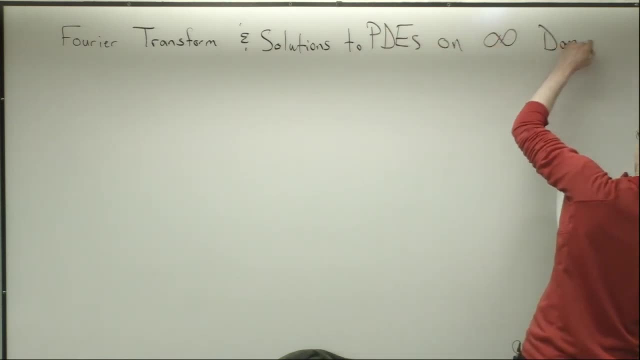 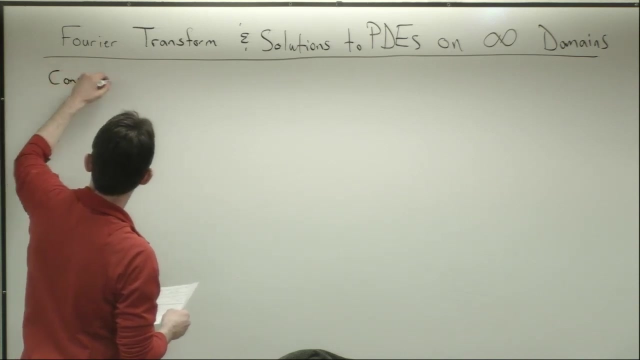 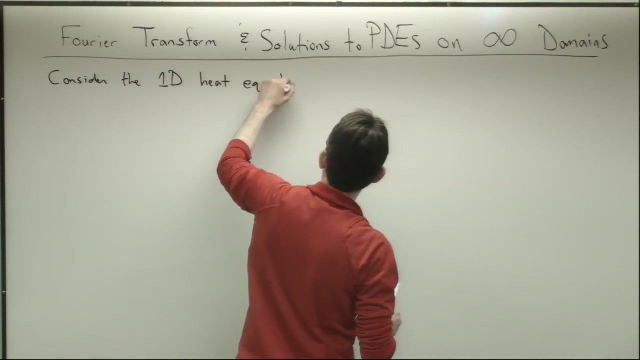 So we're going to solve PDEs on infinite domains And, in particular, we're going to solve the 1D heat equation. Okay, Okay, Okay, Okay. When have we solved the heat equation before? What kind of domains have we solved the heat equation on? 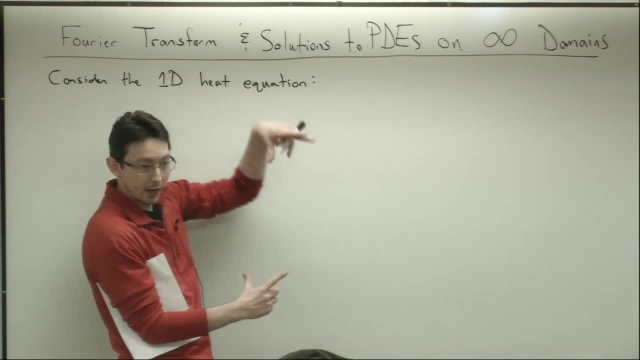 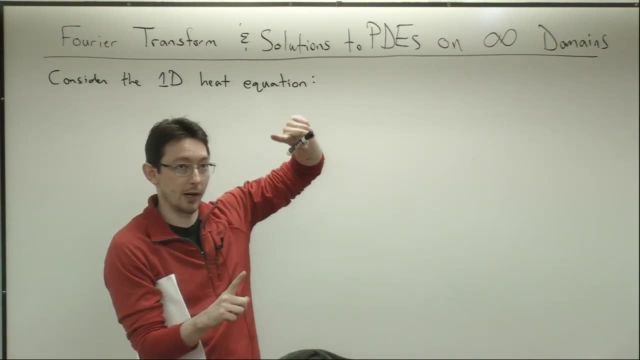 Sorry, Like a defined space. A defined space like a rectangle. I think we also solved not necessarily the heat equation but Laplace's equation on a circle. I think we solved it on a rectangle, with two different types of boundary conditions. 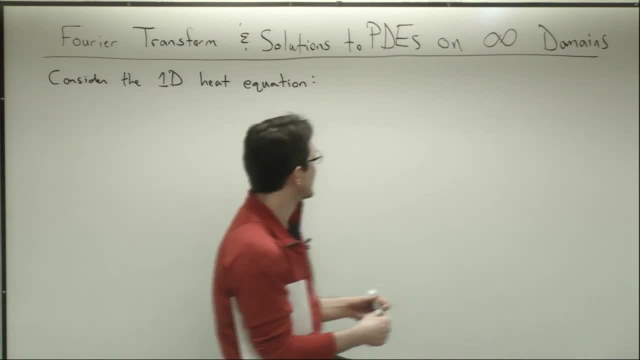 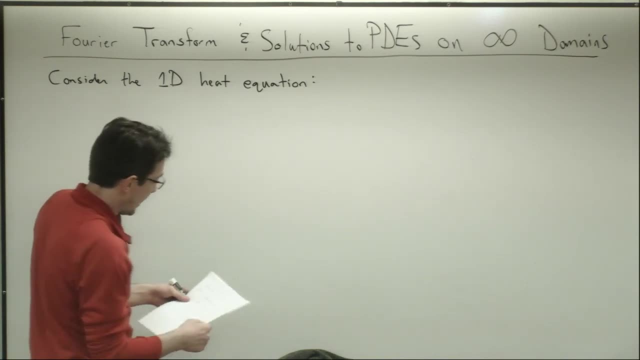 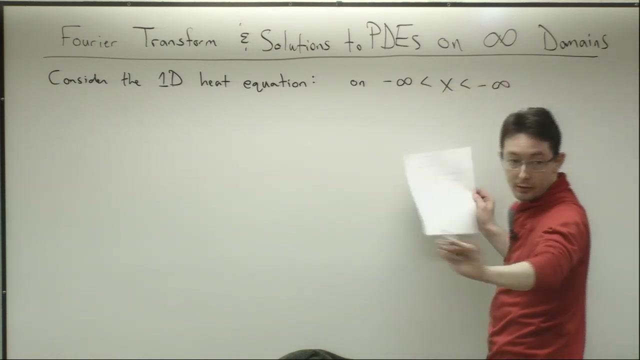 We had fixed temperature and insulating boundary conditions And we also solved it. And we also solved it on like a fixed interval in 1D. okay, a bunch of different ways, Okay. so now we're going to be solving the 1D heat equation on the entire real line. 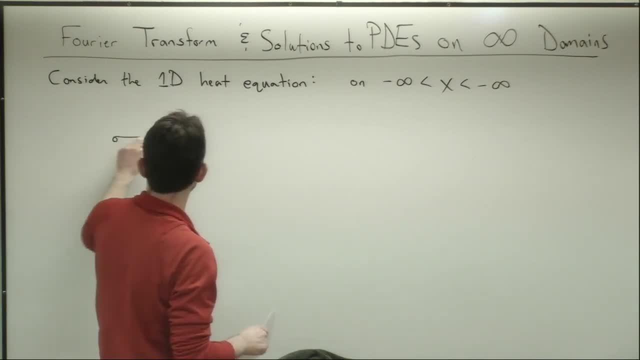 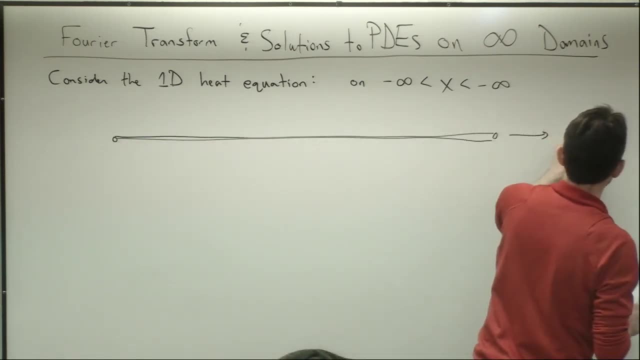 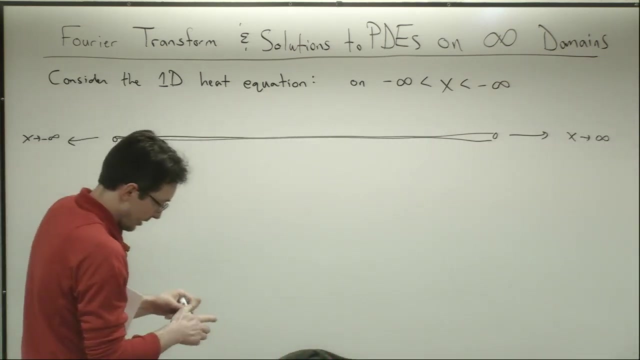 And so the picture that I like to think about this is that we have our very thin but infinitely long steel rod, and this goes to, you know, x to positive infinity, And this also goes x to negative infinity, And I'm going to have some initial temperature distribution. 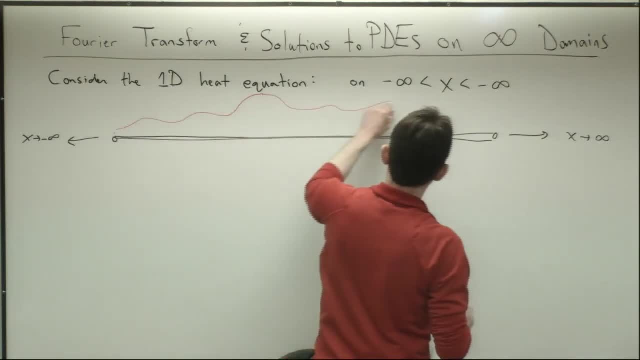 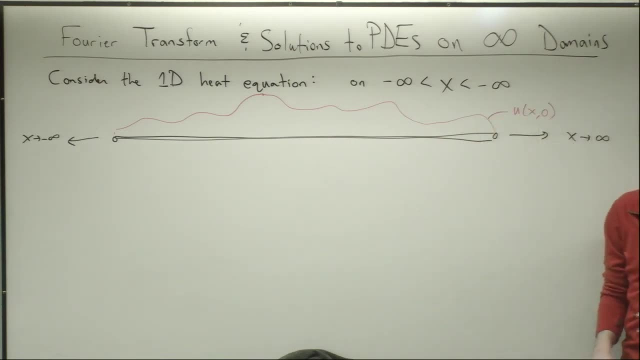 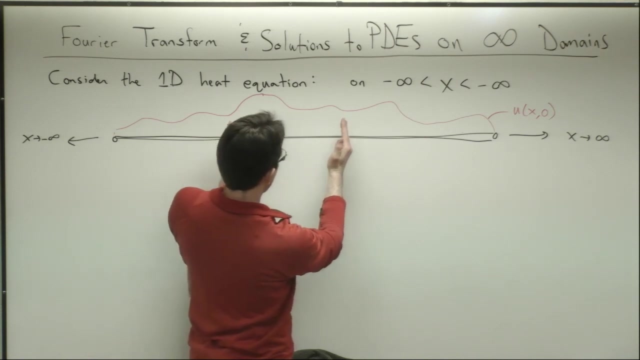 So I have some initial temperature distribution that I'm going to call u, of x at time zero. So I have some temperature at all space but defined at time zero. So if I had my heat equation on a finite piece of steel from zero to one, what other information would I need? 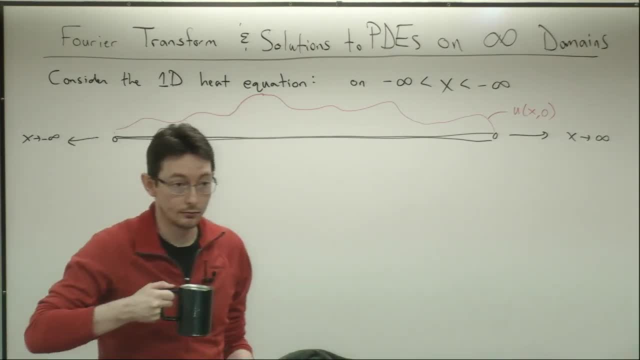 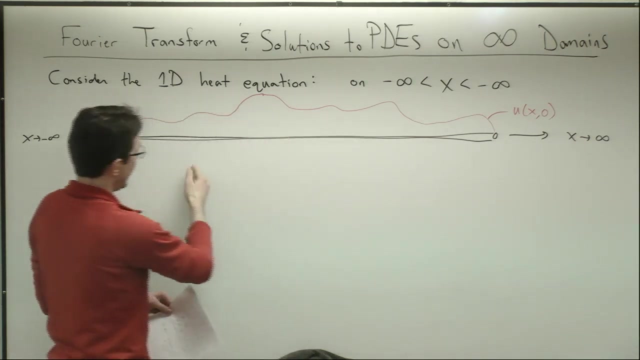 boundary conditions. so what kinds of boundary conditions could i use for a finite length piece of steel? yeah, so i could have something from negative l to l and i could fix the temperature at the end points forever. i could say they're just equal to a and b, or i could fix the flux through the. 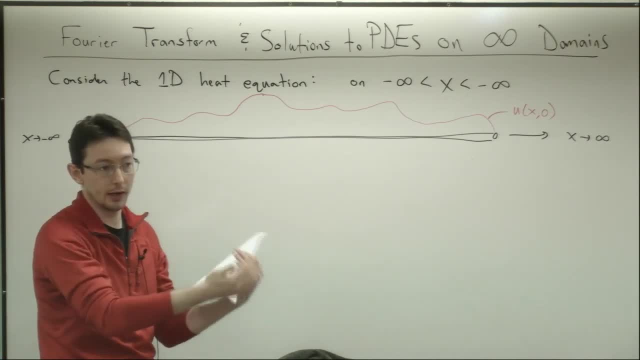 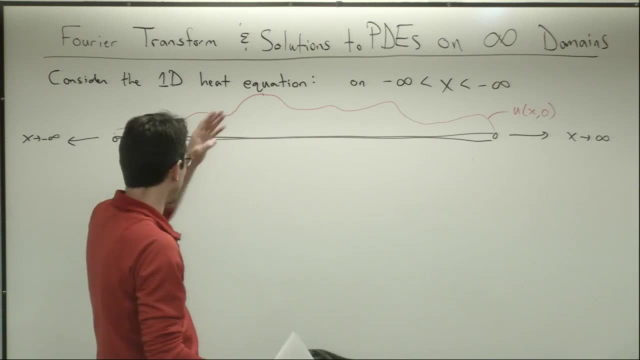 boundary conditions? i could say that they're constantly pouring heat or absorbing heat at a fixed rate, but here, when i have an infinite domain, things are a little bit different. so what are reasonable boundary conditions for this problem? at the kind of infinite ends of this, this rod, what do we think should probably happen? 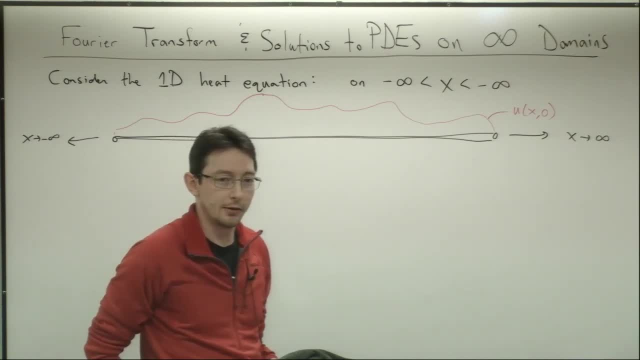 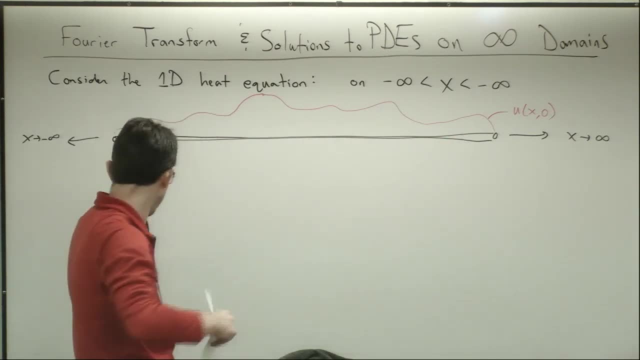 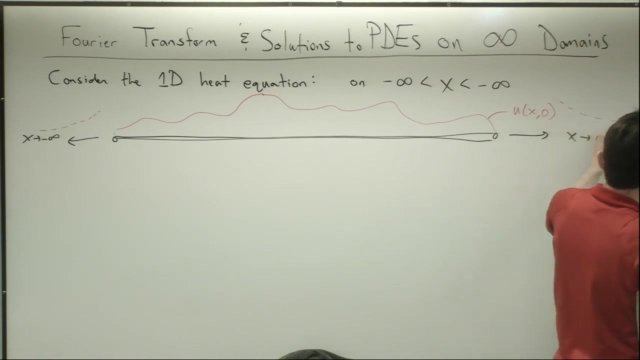 probably go to zero. i don't think it would make a lot of sense to have an infinite um amount of heat energy in this rod, so i want them to taper off to zero. so i kind of have that these you temperature distributions are asymptoting to zero. 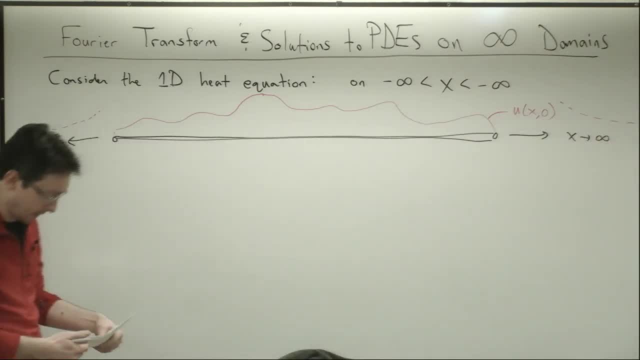 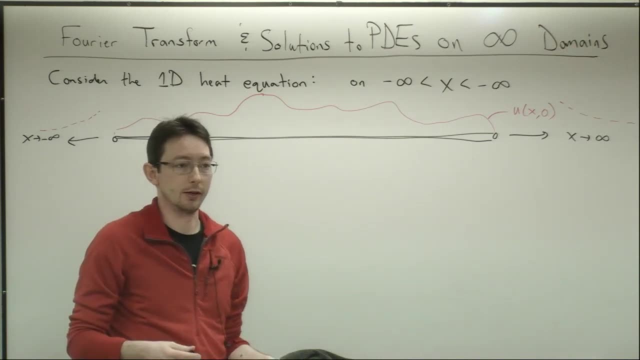 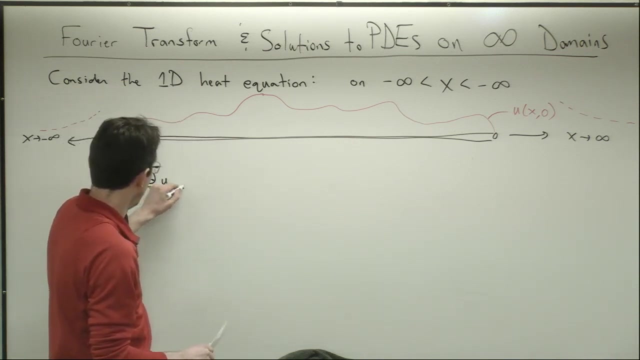 as x goes to plus and minus infinity. okay, good. um, what does our 1d heat equation look like? what is the actual equation? the partial differential equation, right ut. so the first derivative of my temperature with respect to time equals. okay. i have some second derivative of my heat, of my temperature, with respect to x twice, and i have 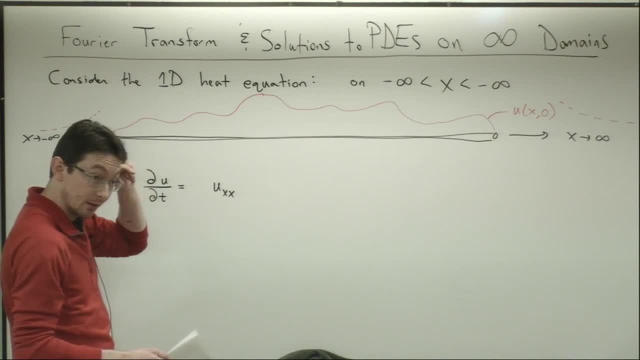 some constant out front. and what can that constant be? has to be positive. so at one of the exercises- i haven't decided if this is a homework exercise or what would be- to try to solve this equation, just like what we're doing, but for a negative thermal constant, things are going to go really. 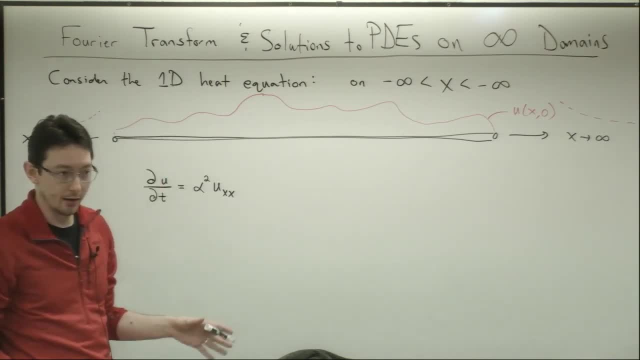 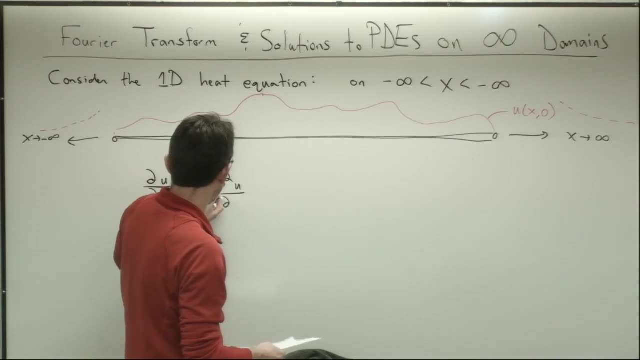 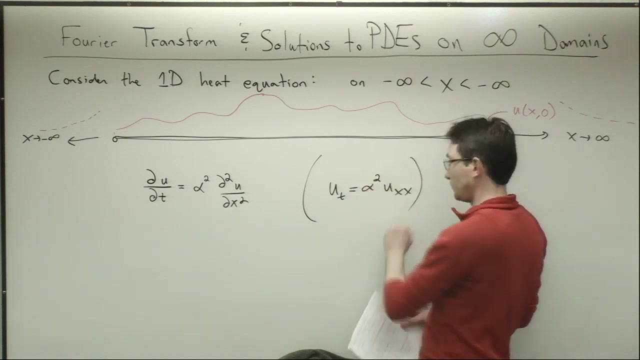 badly. so you need a positive, a positive constant here. uh, do you could have? maybe i should not mix notation. so this is partial squared u, partial x squared. and another way to write this is: you t equals alpha squared u x x k. that's the heat equation. that's always been the heat equation. 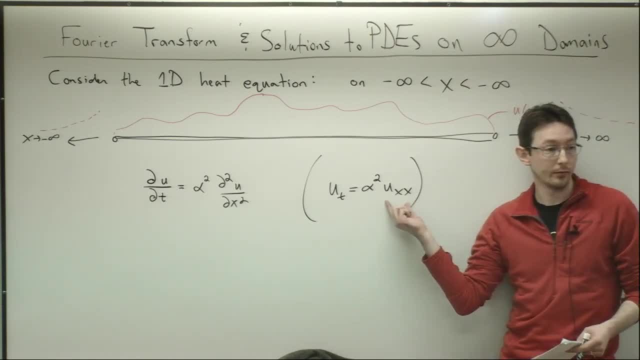 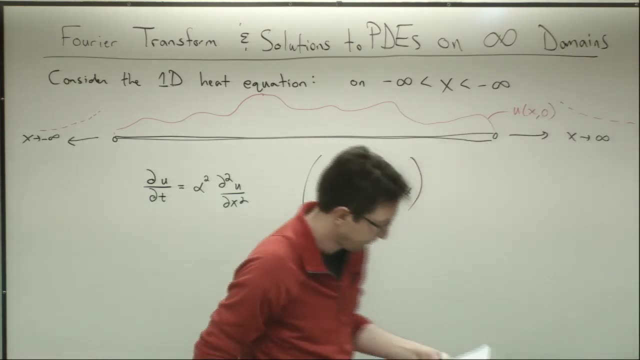 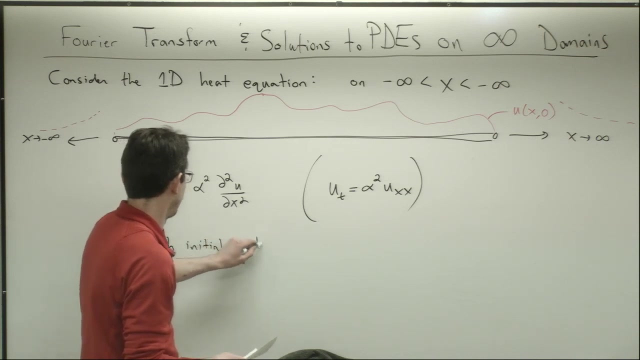 if this wasn't higher dimensions of. at first, a little caution of you which repart you partially, expect social you purple. why y trust partially, partials. easy, as many variables as i have, okay, and i have wislab with initial condition: u of x. at time 0 equals f of x. 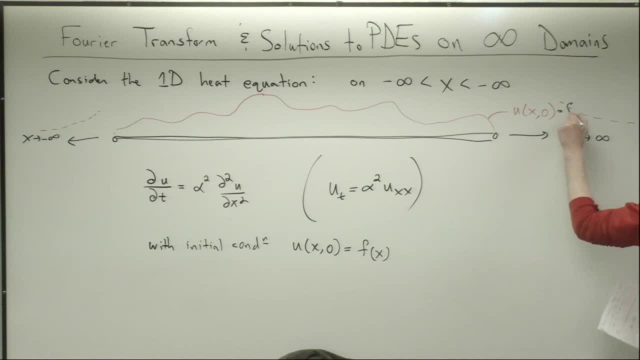 I just have some initial temperature distribution. so this is equal to f of x And then the last thing I need. so I'm essentially writing down a well-posed problem, And so whenever you get a homework problem or an exam problem, you're going to be thinking to yourself. 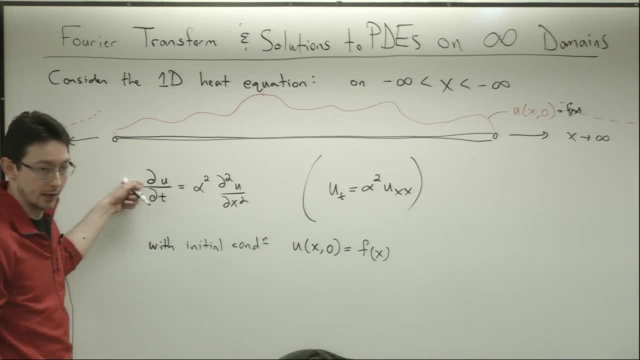 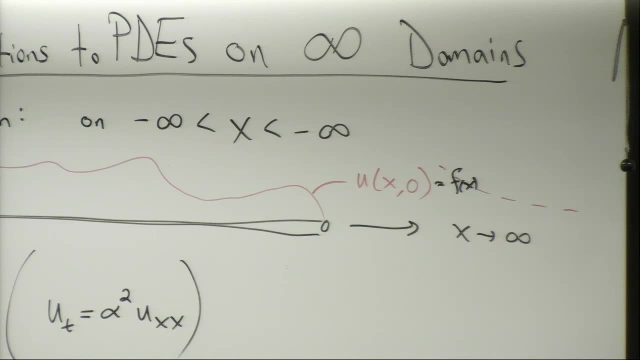 is this problem well-posed? I have an equation- Good, I need an equation- I have some domain that this equation is defined on, and I have some initial conditions and boundary conditions. So my boundary conditions are essentially- I'm just going to write this in shorthand- 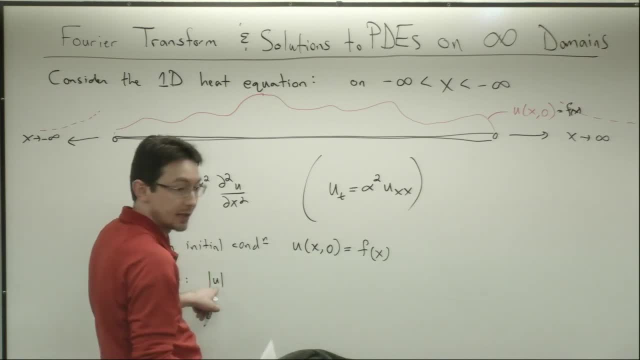 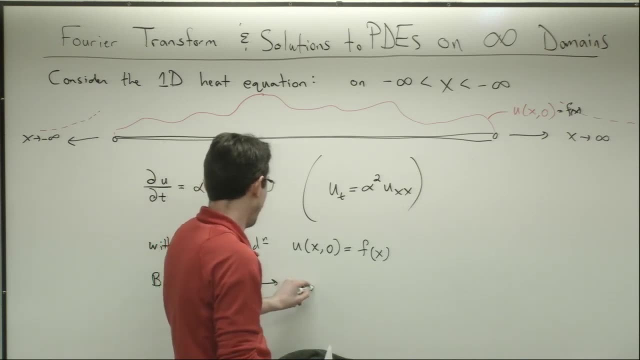 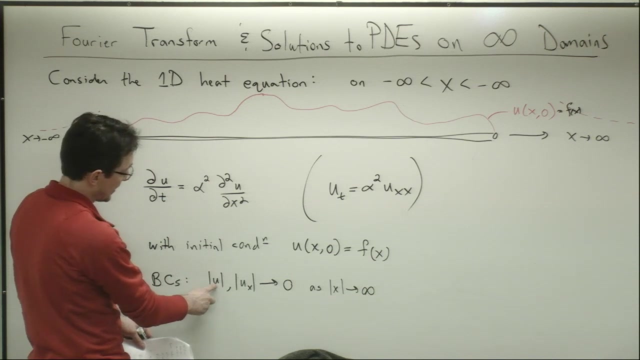 So we have u the magnitude of my temperature and also the magnitude of the first derivative of my temperature go to 0 as my spatial variable goes to infinity. This is just shorthand to say that this could be the absolute value of these- goes to 0 as x goes to plus or minus infinity. 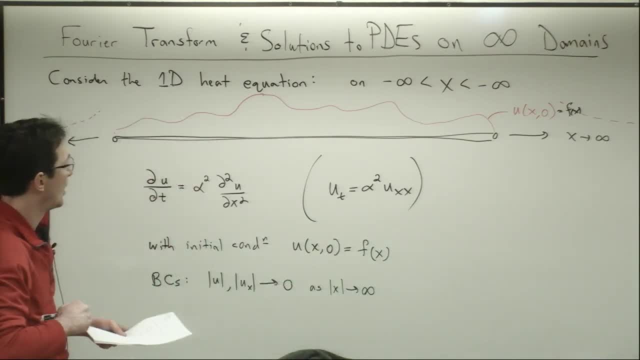 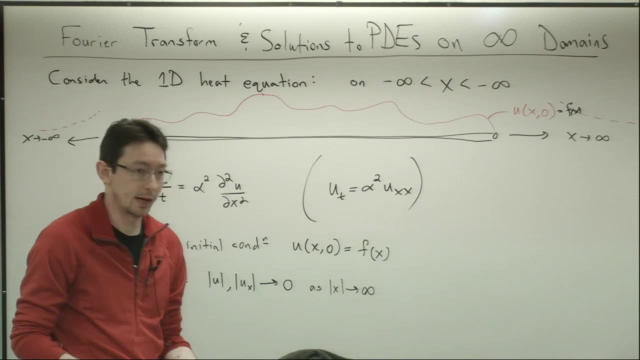 as the magnitude of x gets large. OK, so there are a couple of ways to solve this problem. One of the things we've already learned is separation of variables, So separation of variables is probably the most robust way of solving any linear partial differential. 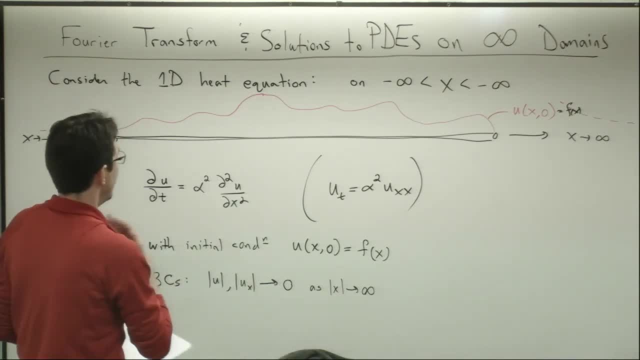 equation. We can almost always do it. It makes a lot of sense And it's clear. It's kind of a procedure where you can solve the system in terms of these eigenvalues. The second way we can solve this problem is to take the Fourier transform of this equation. 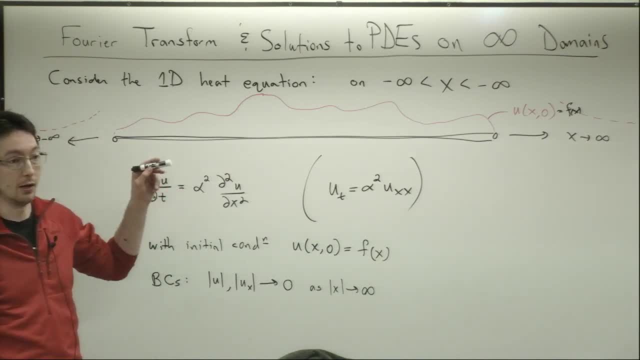 to take the Fourier transform of our temperature with respect to space x. So that's what we're going to do today. So I think you should try to solve this using separation of variables and see what you get. It would be a pretty simple 30 minute exercise. 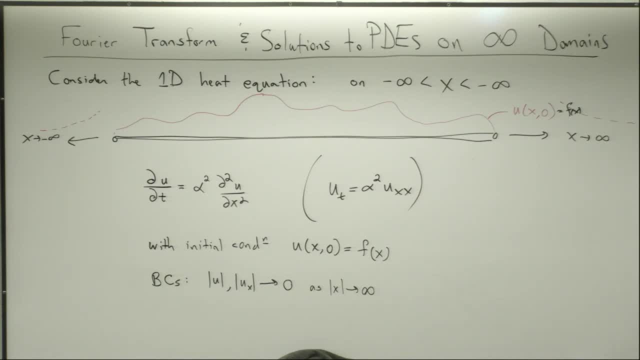 and it's a good thing to try, Probably 30 minutes. 30 minutes if you don't care that much about all the signs and all the details, but you can get a feeling for it. OK, so we're going to Fourier transform. 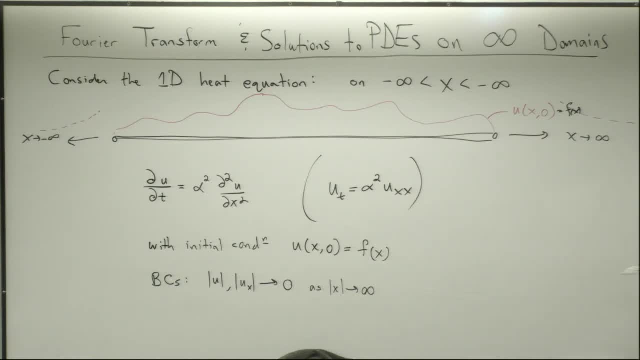 And we're going to Fourier transform in space. OK, so we have an infinite spatial domain, from plus and minus infinity, And so we're going to Fourier transform in space. because we know our Fourier transforms are defined on infinite domains, We're going to Fourier transform in x. 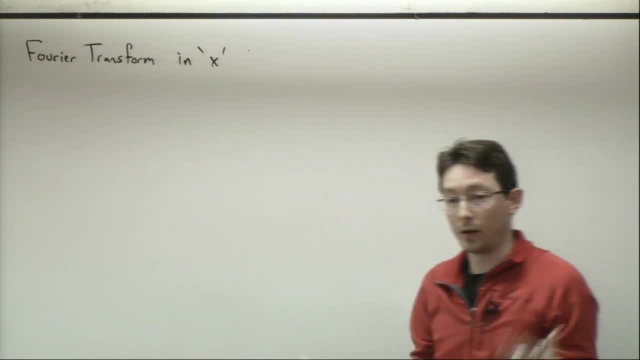 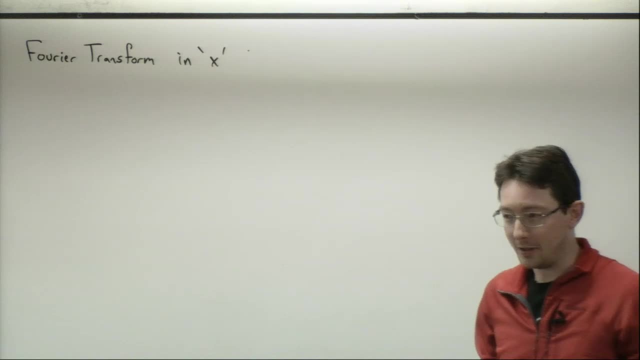 OK, And what we're going to get? we're going to turn our PDE into an ODE, which is awesome. We know how to solve ODEs. Remember, last quarter was way easier. All of the ODEs were a lot simpler. 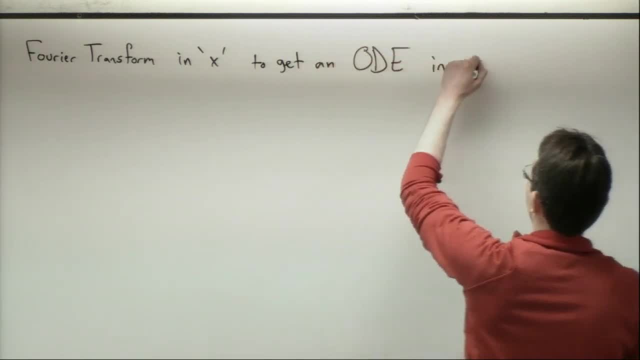 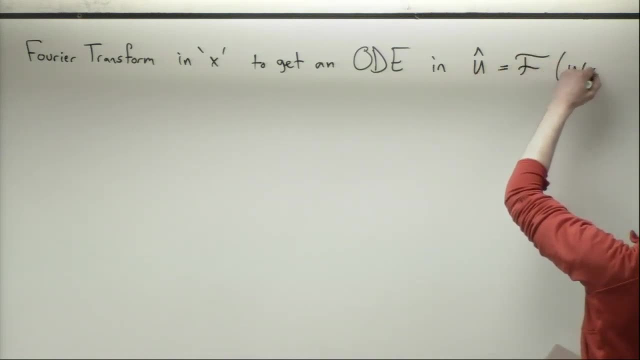 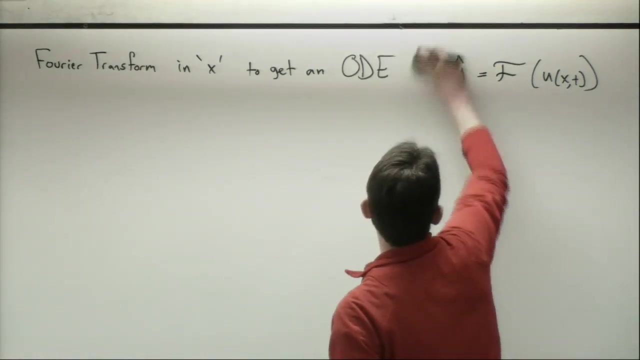 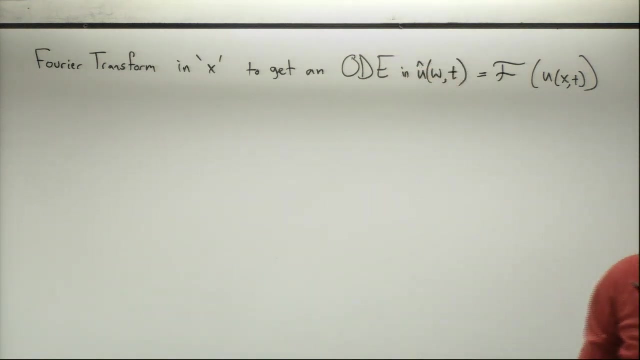 So we're going to get an ODE in u hat where u hat equals the Fourier transform of u of x in time. OK, Maybe I should be a tad bit more explicit: u hat of omega and t right, My spatial variable x, when I Fourier transform. 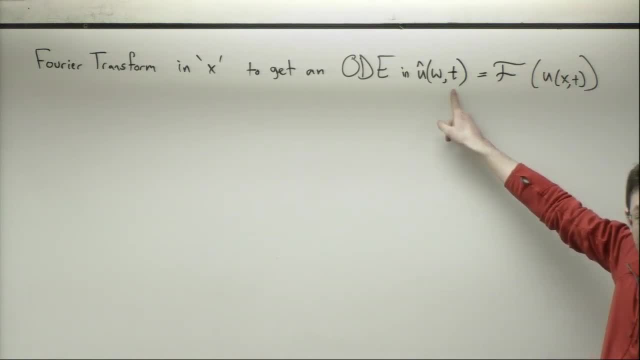 turns into a frequency variable, omega, But it's still a function of time. I'm not Fourier transforming in time. Time is a constant with respect to this Fourier transform. OK, Make sense so far, And please interrupt at any point. At any point, this is important to see how this all goes. 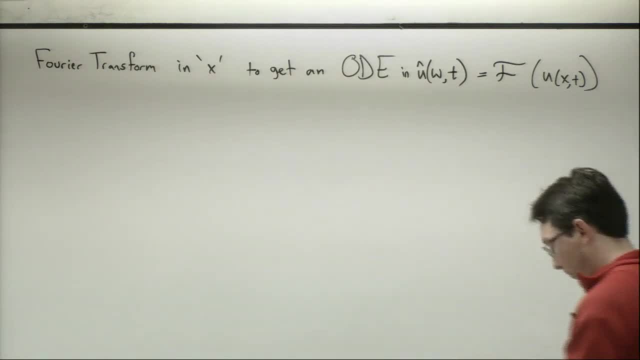 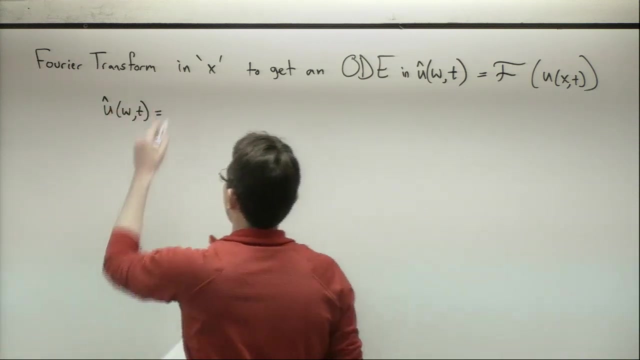 So I want you to interrupt if you have questions. OK, I should probably write down a Fourier transform integral at some point, because I just realized I didn't do that. So I have u hat of omega. t equals the integral from minus infinity to infinity of my function, u of x and t. 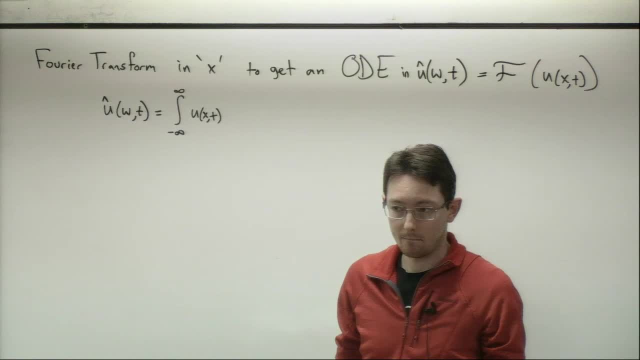 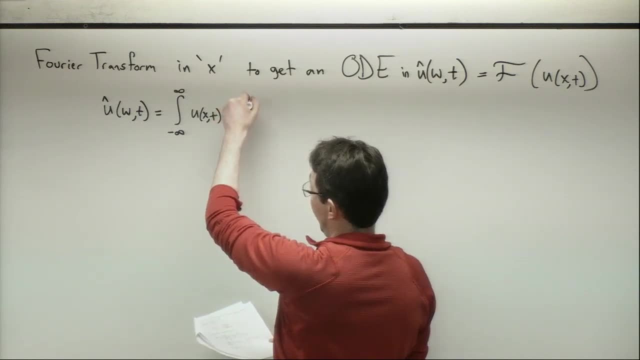 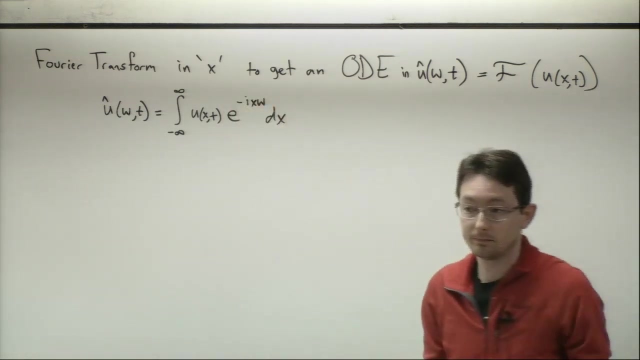 times what. What do I do to Fourier? transform u e to the? I believe it's minus i x, omega, dx. Wikipedia says there's a minus sign here And my old math teacher, Phil Holmes, also says there's a minus sign here. 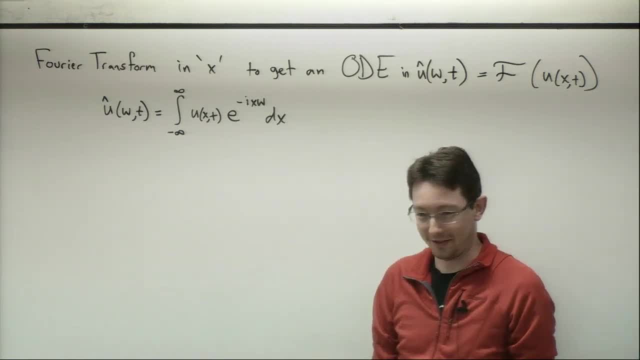 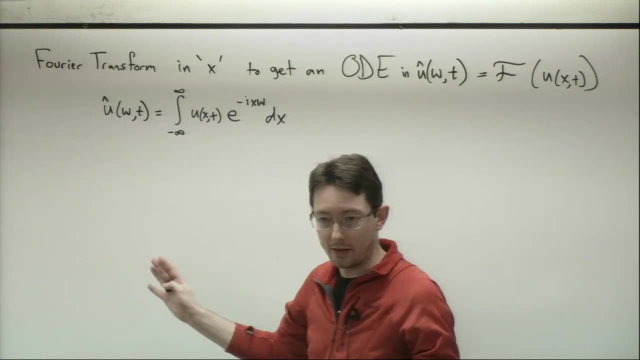 The book I was using does not have a minus sign here, and it's wrong, I think, So let's just go with this for now. So that's the Fourier transform. We derived this as the limit of a Fourier series, as l goes to infinity. 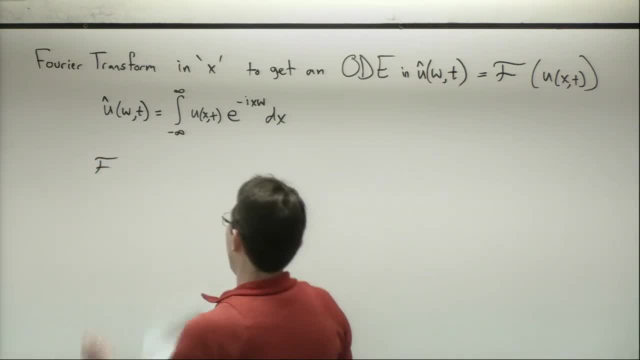 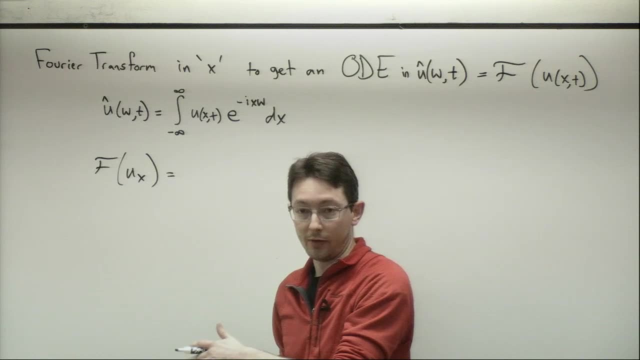 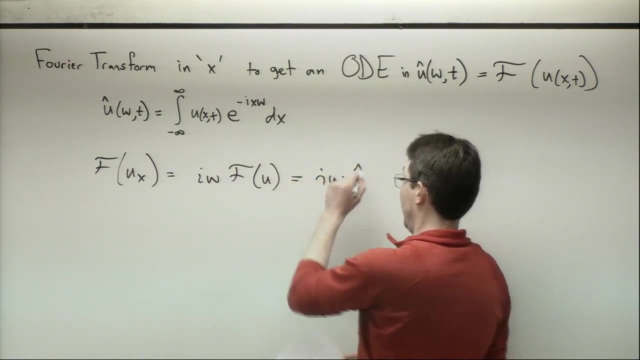 And we also showed at the very tail end of lecture 15 that the Fourier transform of ux is equal to i omega times the Fourier transform of u. So that's just i omega u hat. Awesome, That's way simpler. At least we think it's going to be. 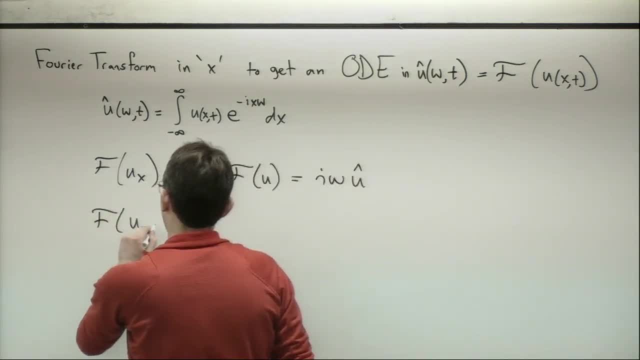 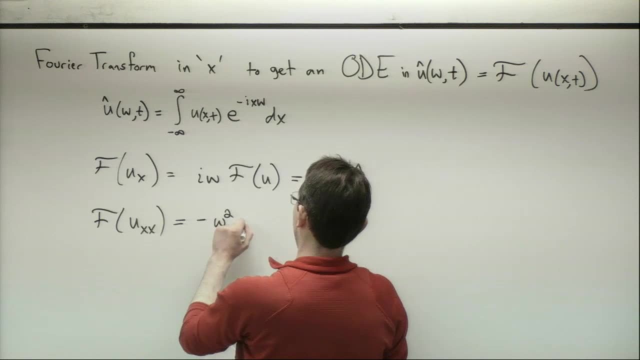 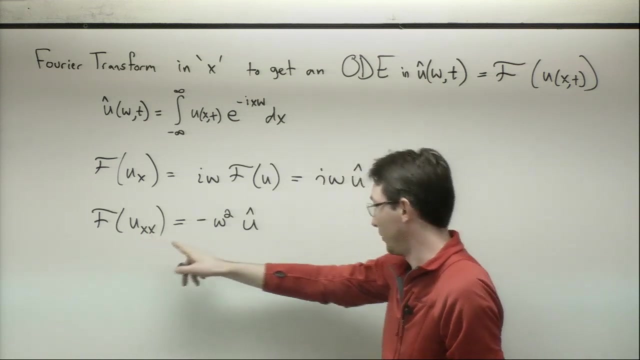 It's going to be way simpler. So the Fourier transform of uxx is just i omega squared, which is minus omega squared u hat, And the Fourier transform of uxxx would be minus i omega cubed. Four x's would be plus omega to the fourth, and so on. 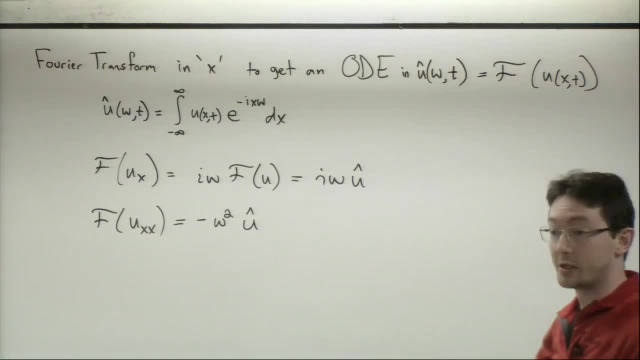 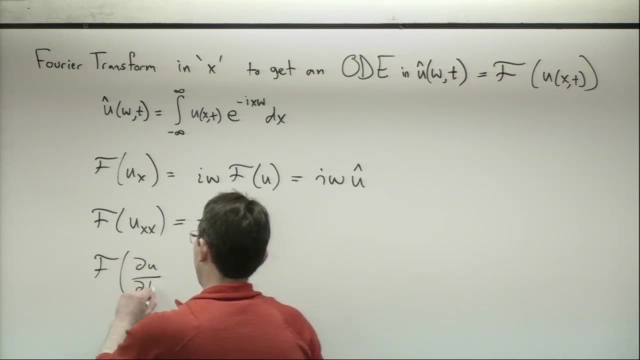 So this just multiplies i omega every time I take a derivative, which is a very nice property. And the last thing I want to talk about is this: The last property is that the Fourier transform of partial u, partial t, Remember this entire Fourier integral. 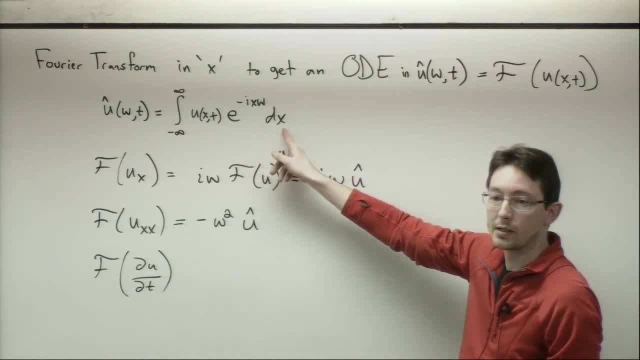 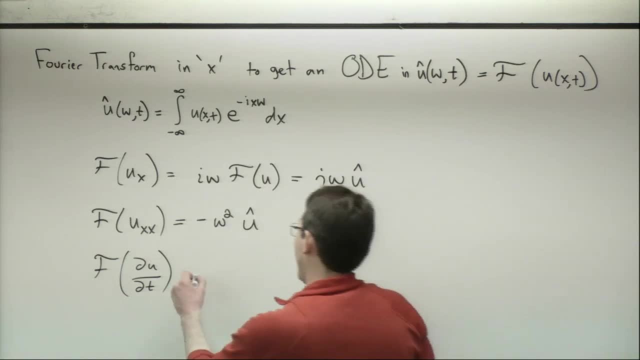 is purely with respect to x, And so time can be considered a constant with respect to this integral in x, And so this partial can pop out, And this equals partial t of the Fourier transform of u, which is equal to u hat sub t. 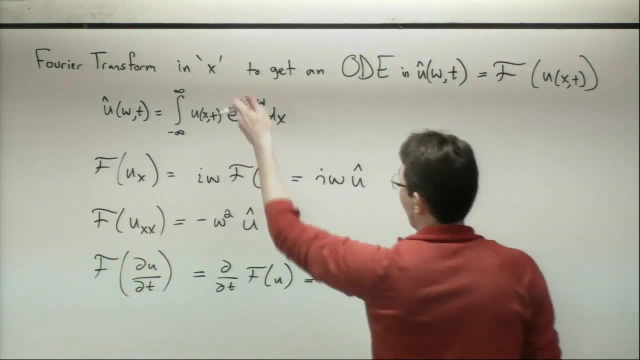 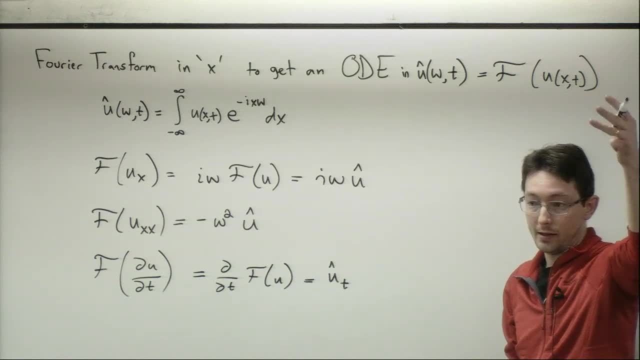 OK, So this is great. What we have here are the Fourier transforms of all of our variables of interest. We can Fourier transform u, ux, uxx and ut, And what we get is a way to transform our partial differential equation. 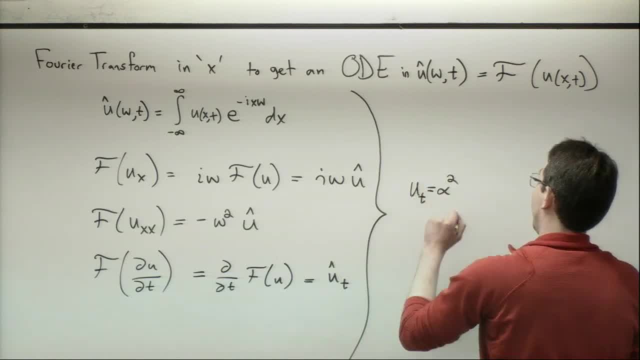 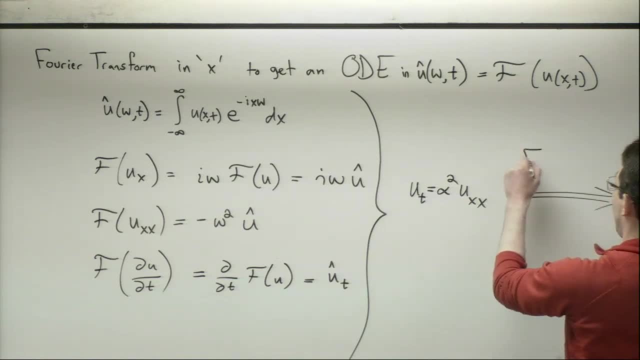 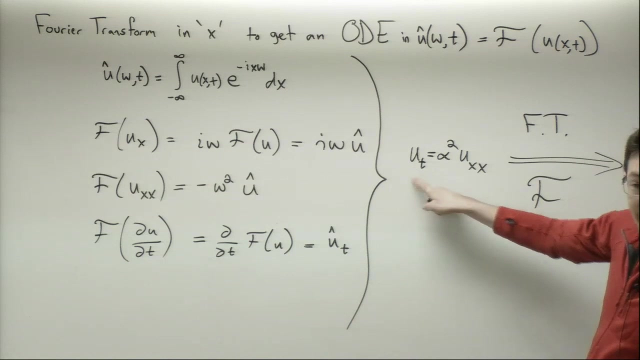 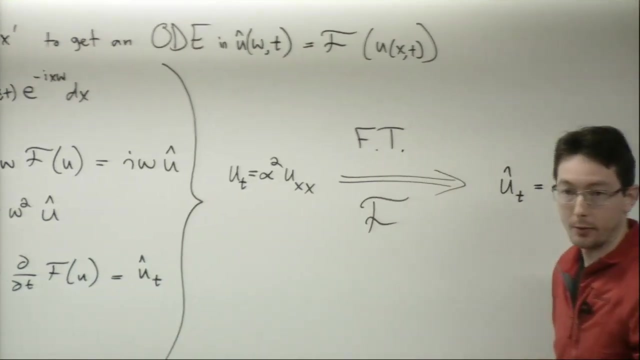 So we have ut equals alpha squared uxx And we're going to do this Fourier transform And what I'm going to get is u hat t equals constants Just pop out of the Fourier transform. The Fourier transform is linear, So the constants pop out. 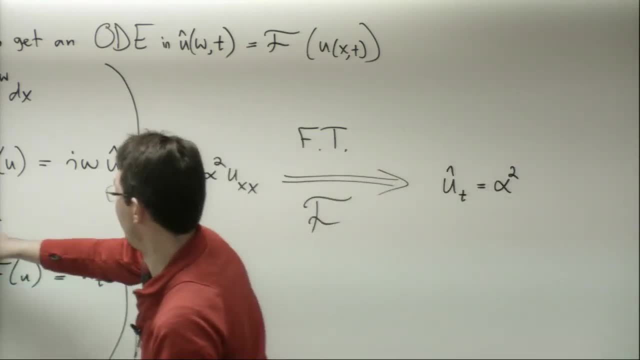 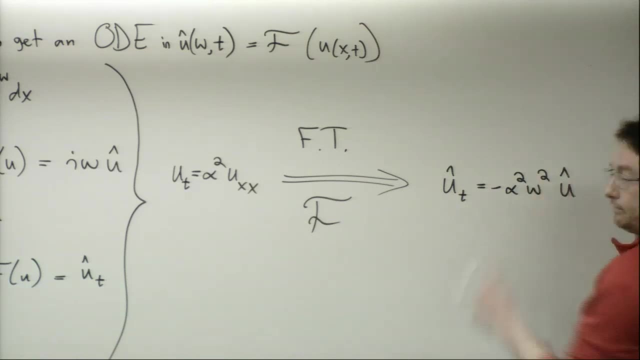 Alpha squared times minus omega squared. So minus alpha squared omega squared, u hat Right. So uxx is just minus omega squared u hat OK. This is amazing. We just went from a PDE to an ODE, right? There's only one partial derivative in this. 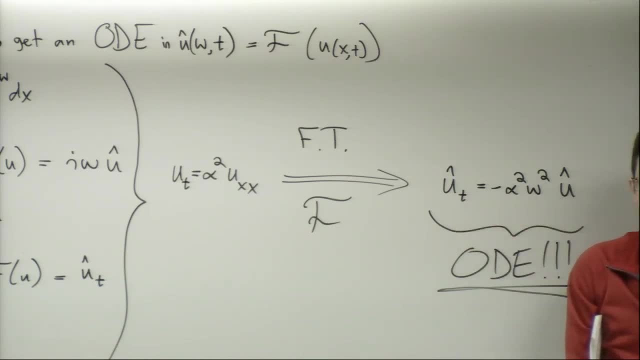 It's with respect to time. There's no partial x's anywhere. So this is just an ODE, a first order linear ordinary differential equation in u hat. That's with respect to time. OK, And we know how to solve these. 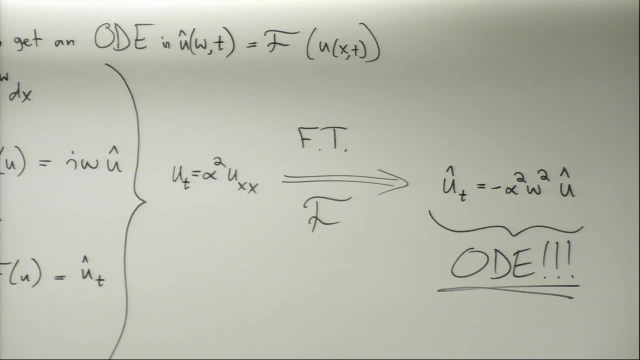 OK, questions about how we did that or why this is an ODE or anything. Yeah, The first line of derivatives, the Fourier transform of u, up here. I don't know how to duplicate that, So we got this from Lecture 15.. 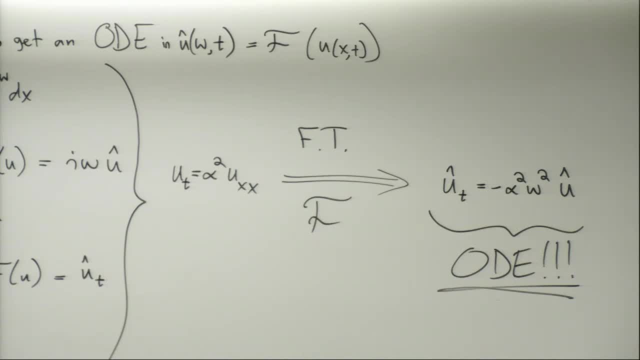 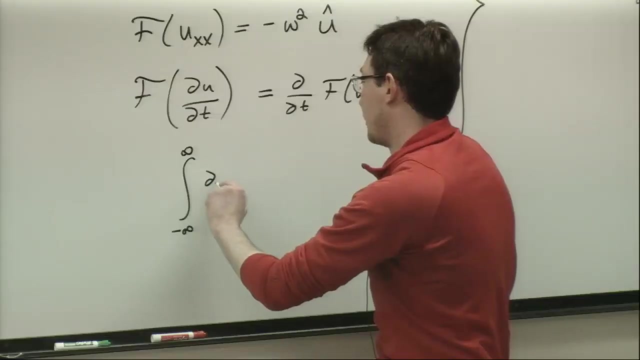 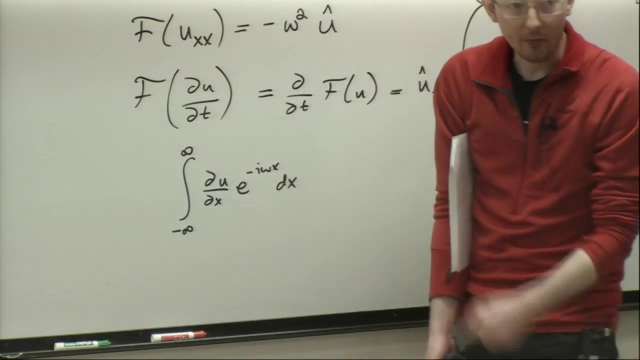 And essentially we did integration by parts. so this is the integral of. you know you write this as, what is it? so the Fourier transform of ux, you have this integral minus infinity to infinity of partial, partial x, of u, e to the minus i, omega, x, dx, and this is a terrible. you know we always call them u and dv. 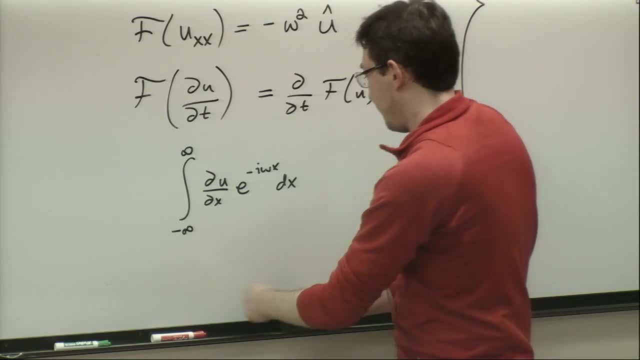 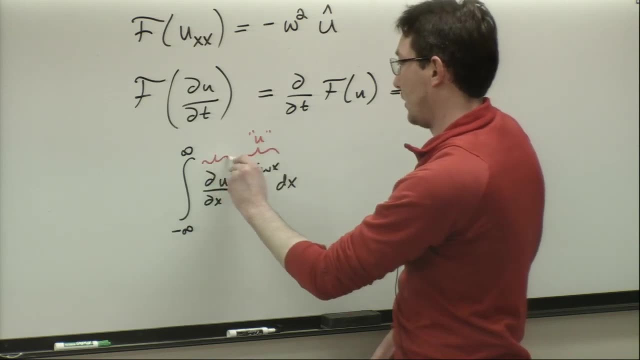 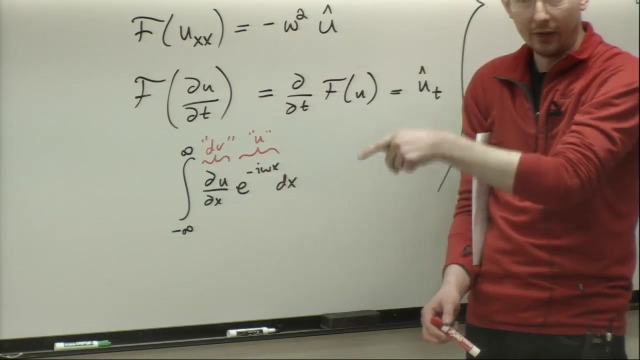 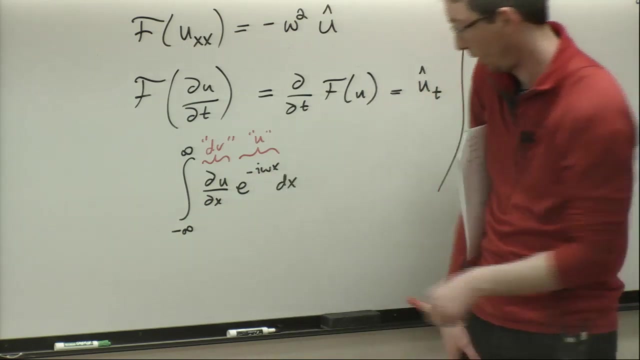 but this is called u, so this is really confusing. but you would say that this is the integral of u times dv. right, this is a differential, and then that would equal uv minus the integral of vdu. and everything just pops out because du has a minus i omega out front. okay, and it would be a 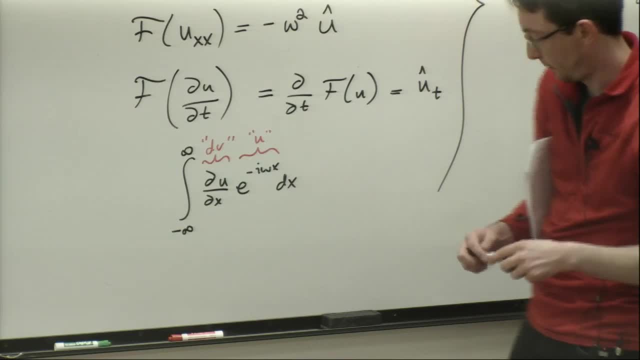 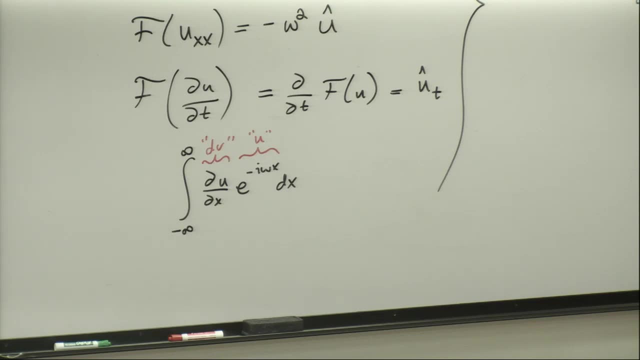 minus, minus i omega, because it's minus the integral of udv. okay, okay, so that's how you get the this property. okay, good question. um, it's always a little difficult when there's a week between lectures, um, and this is a really, really important property, so i'm glad, glad you asked, okay, uh, other questions? 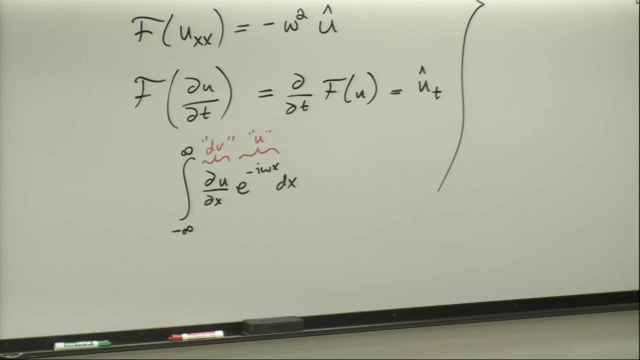 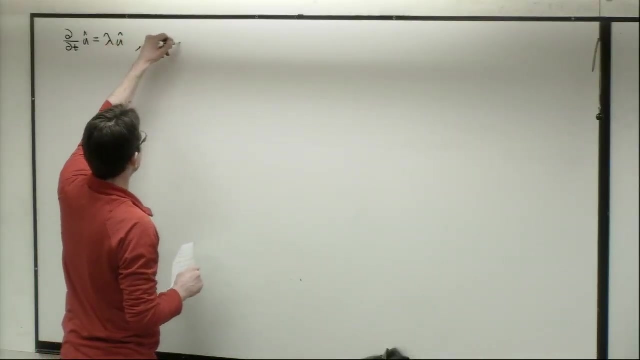 make sense so far, okay. so let's look at our ode. we have partial, partial tertiary t of: u hat equals lambda times u hat, where lambda equals minus alpha squared, omega squared. those are numbers as far as time is concerned. those are numbers, okay. so this is what my ode looks like: u hat dot equals lambda u hat. 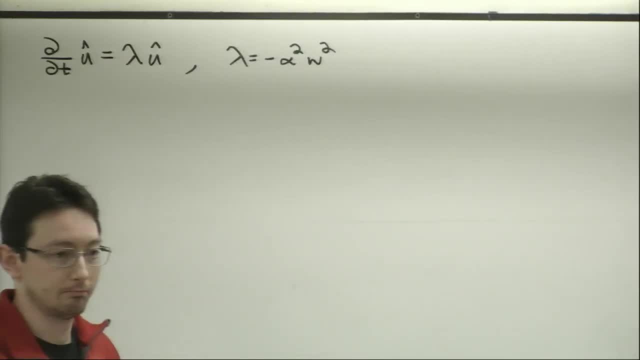 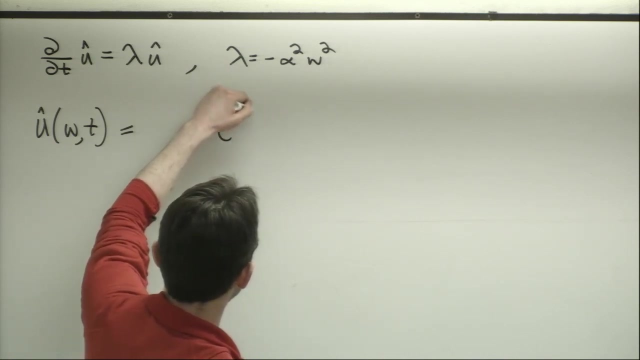 and what's the solution? So u hat of is a function of omega and t and it equals what e to the lambda t, e to the lambda t, that's e to the minus alpha squared, omega squared t times. u naught which is and what's the naught. 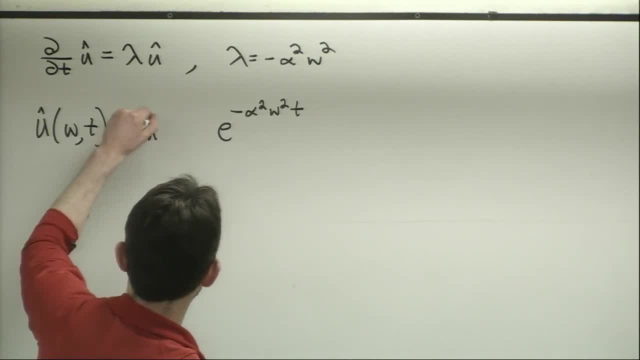 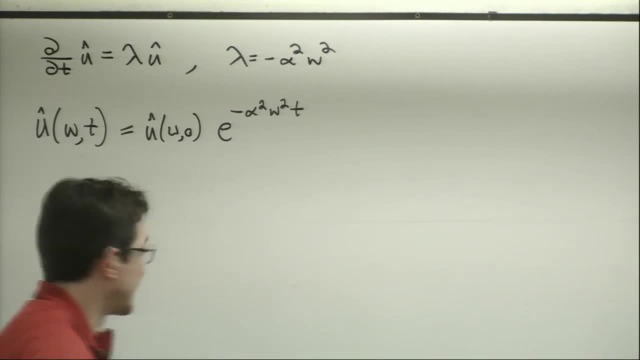 It's zero in time. So that's u hat of omega comma, zero in time. That's the solution. Let's see if this is what I'm supposed to circle. This is what I'm supposed to circle. This one is important, Okay. 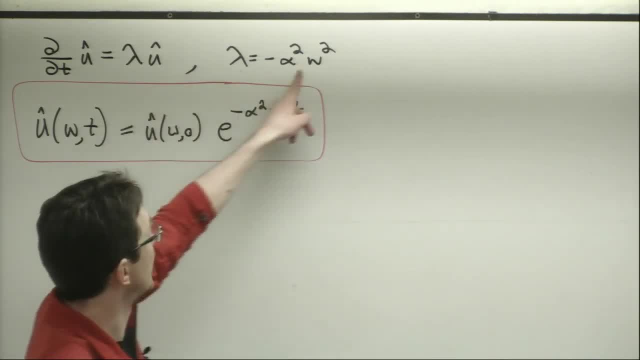 This is incredibly simple. We get an ordinary differential equation in every frequency, For every omega. this is an ordinary differential equation. That's just a number. This is just an ordinary differential equation and this is the solution And it's solution. 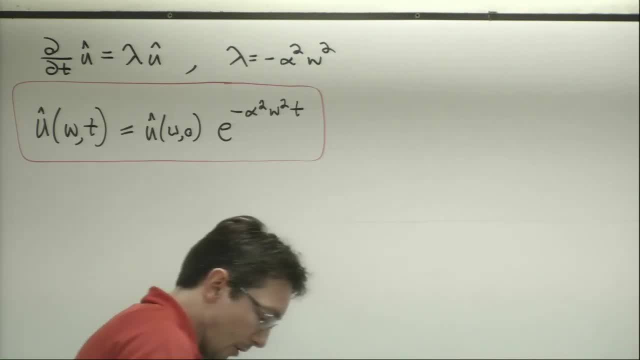 It's a function of omega, but that's totally fine. Okay, So how do we get u hat of omega at time zero? How do we get u hat of omega at time zero? Sorry From the definition, Yeah From the definition. 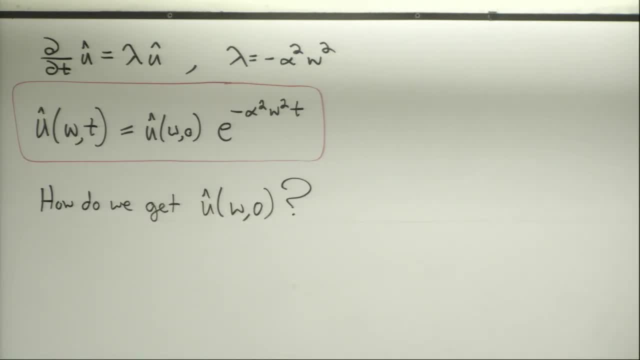 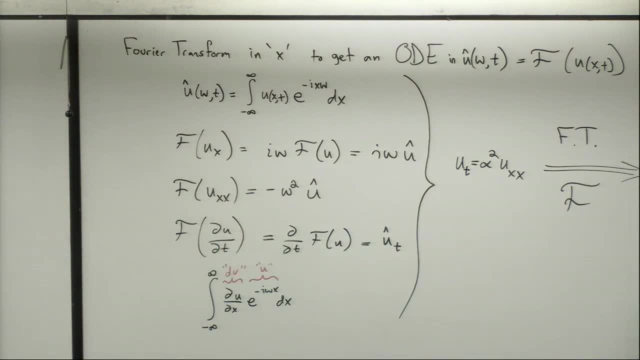 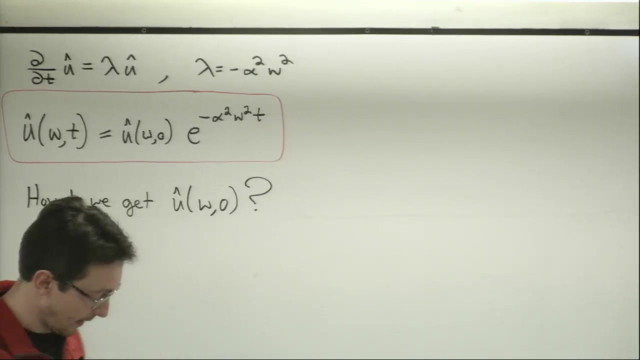 Why not Good? Why not just from the definition Plug in time zero? That seems totally reasonable. At time zero it's still a function of x. I can still Fourier transform it. So u hat of zero and omega a function of omega at time zero. 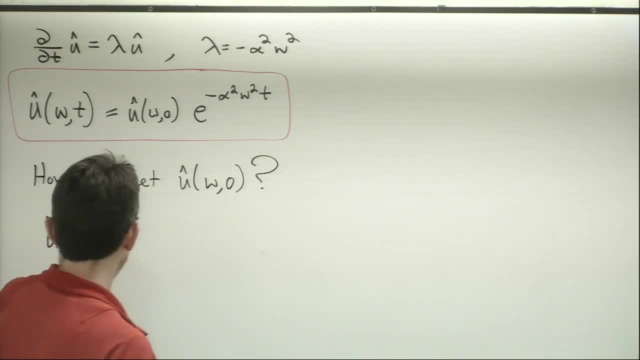 is just the Fourier transform of my initial condition. This is just equal to the Fourier transform of u of x at time zero, which is equal to the Fourier transform of f of x, this little function f of x, and if we want to be cute, we can call it f hat of omega. 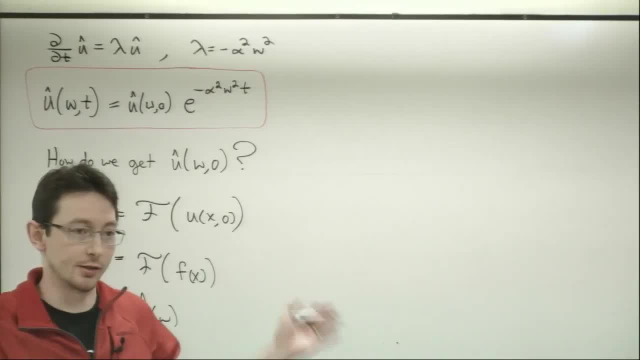 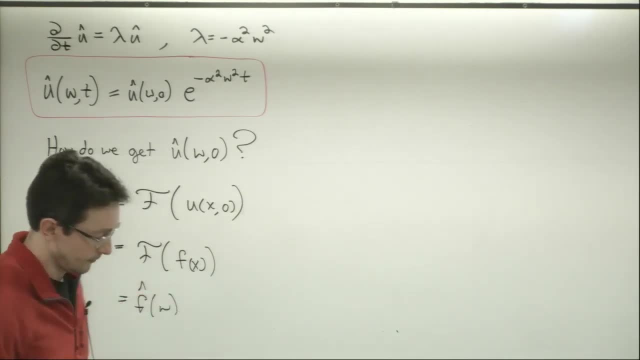 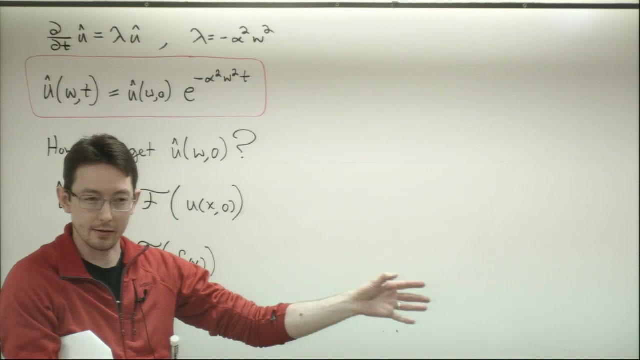 that's totally fine. the Fourier transform of my initial conditions is just f hat of omega. okay, this is wonderful. we have a solution to our partial differential equation, but we're stuck in the frequency domain. we have a solution, but it's in terms of omegas and we live in space. we live in x's. 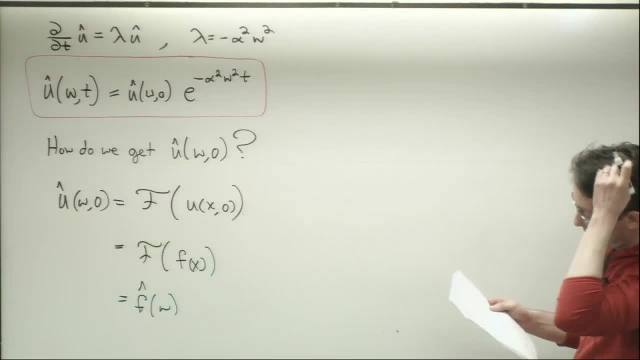 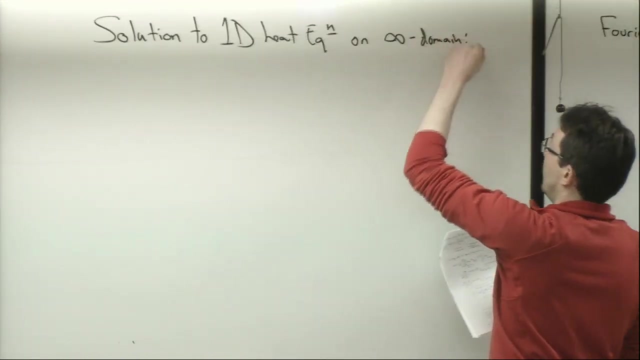 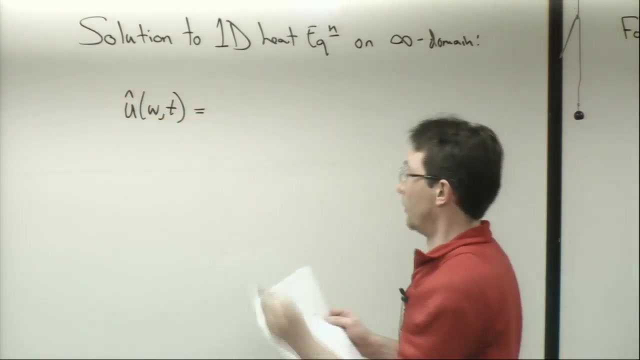 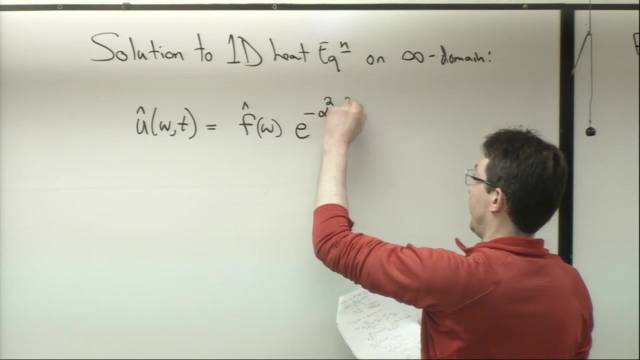 so let's just write this out and get back. so the solution to the 1d heat equation on infinite domain is the following: we have u hat of omega and t equals f hat of omega times e to the minus alpha squared omega squared t. okay, I'm going to be a little bit slow here. 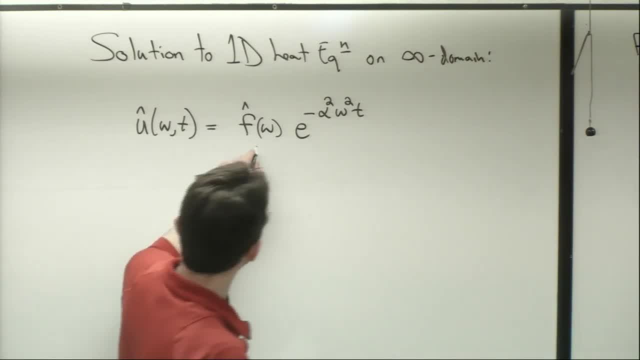 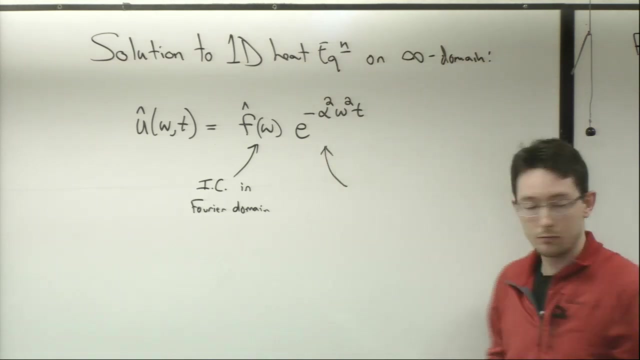 because I want to start building up our physical intuition for what the solution means. okay, so this is just our initial conditions. in a Fourier coordinate system, in Fourier domain, what does this function do? what does this function even look like? exponential decay of? so what do we think of this as a function of? 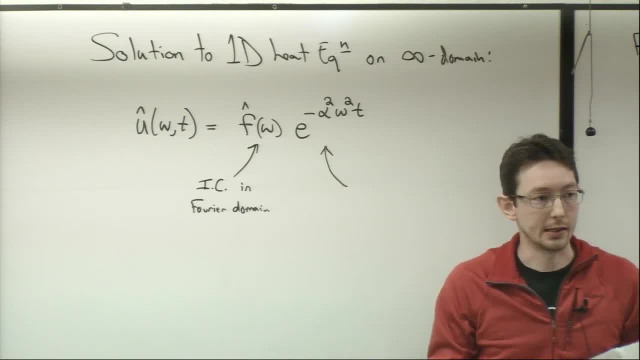 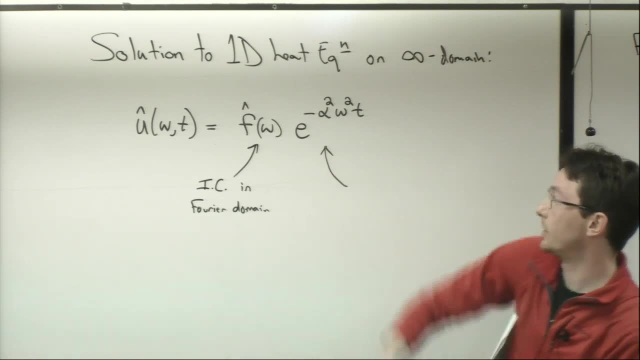 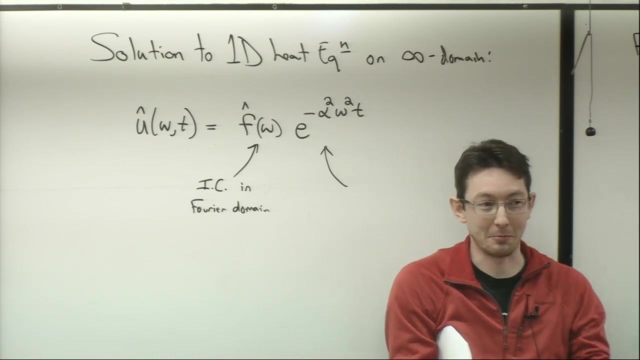 what's this? a function of frequency and time. let's think of it mostly as a function of frequency, and that function of frequency changes in time. okay, so this function of frequency is: does it have a special name? hint, I visited his birthplace last week. 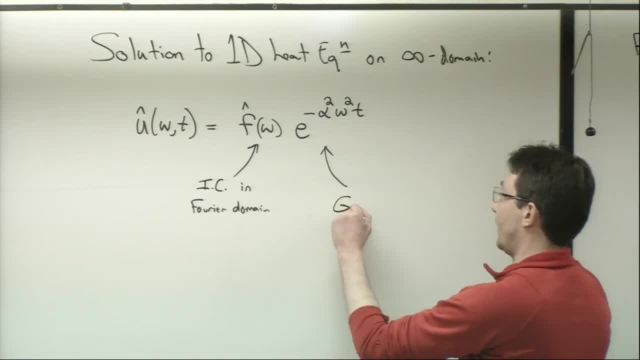 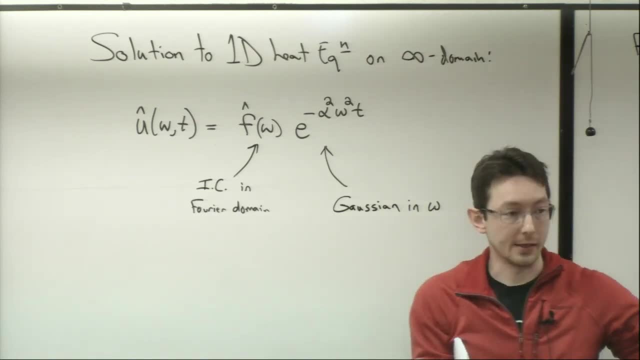 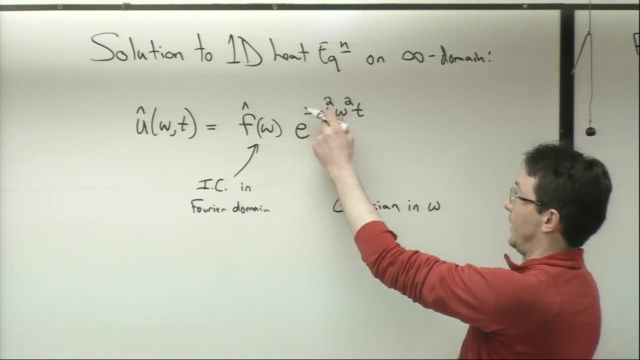 so this is a Gaussian. okay, we have a Gaussian and this is a Gaussian in omega and the variance of this Gaussian spreads out and increases with time. the variance is given by the square root of minus alpha squared t, so I can kind of rewrite this as e to the minus alpha squared t. 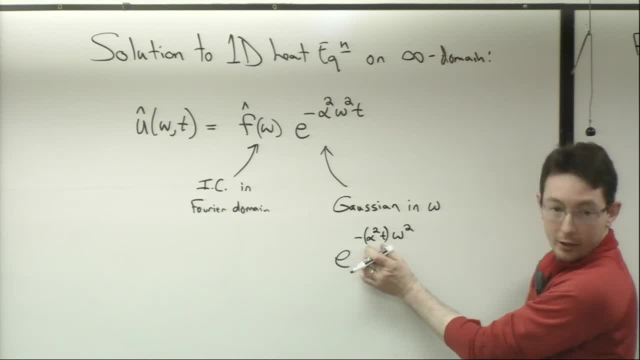 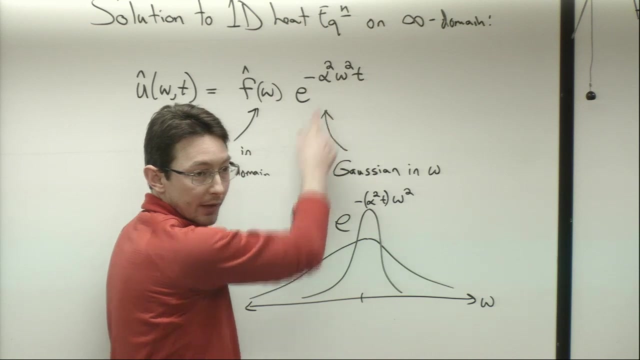 omega squared and this is related to time and this is my equation, okay, so to my variance, and this is my frequency variable. So this is a Gaussian in omega and it spreads out as time increases. You can plot this, Plot this in MATLAB and you'll see that it's a Gaussian. 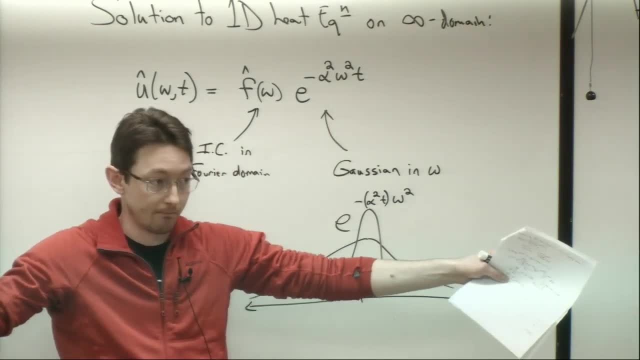 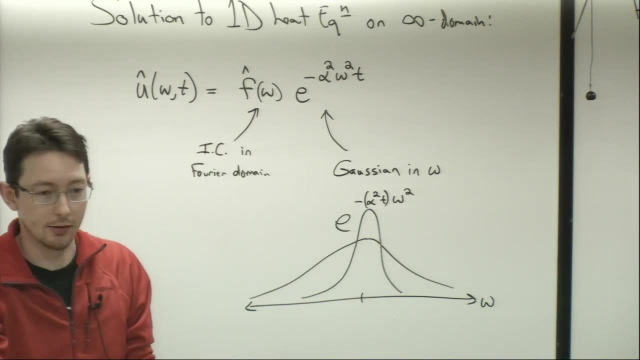 It's a bell curve and it spreads out as time increases. OK, cool, So what's happening? is that another way you can think of this. you said exponential decay, and you're absolutely right that this is an exponential decay in time. 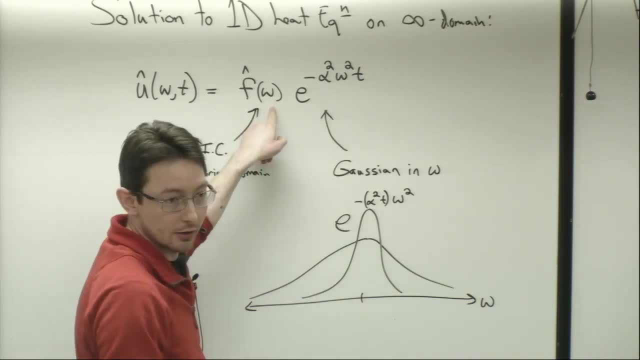 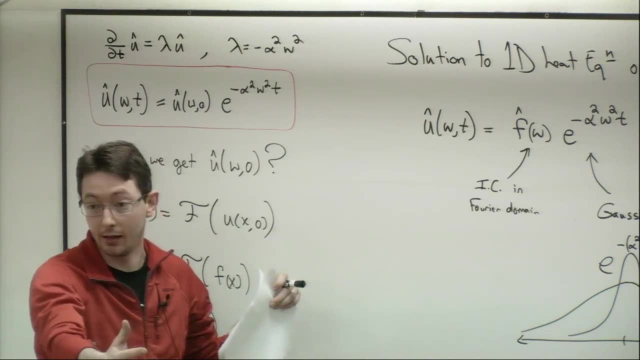 And what that means is that all of my frequencies of my initial condition are decaying. I had this nice initial condition distribution. I could write it in the frequency domain by taking a Fourier transform and all of those frequencies are dying out in time and they're 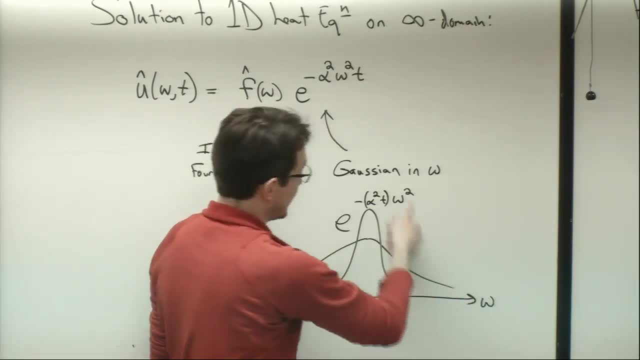 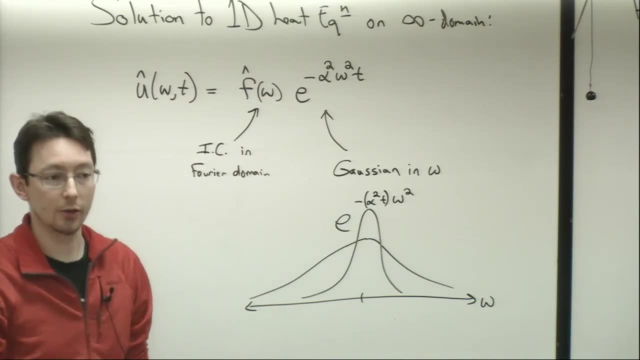 dying out at different rates. Some of them are dying out faster, Some of them are dying out more slowly. OK, so what's happening is that the heat equation, the solution of the heat equation, is damping out. It's killing all of the frequency content. 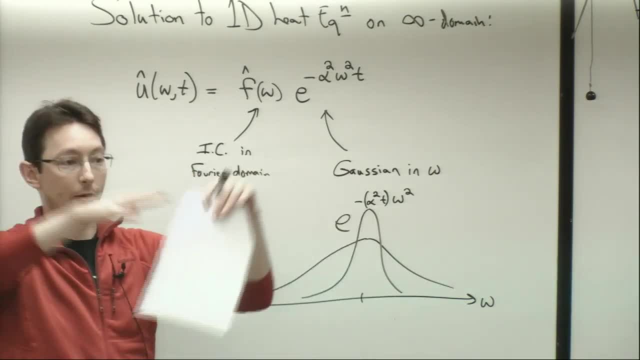 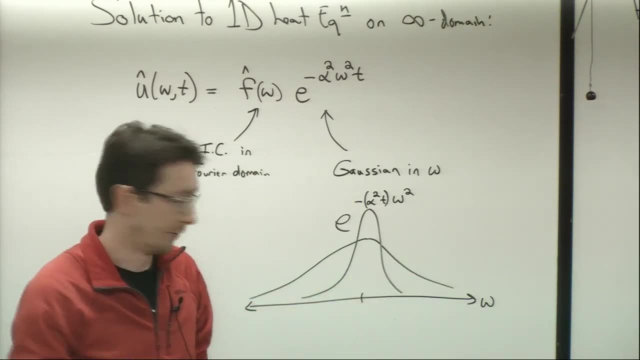 of my initial conditions. All of the variations are getting spread out uniformly until eventually I'm going to have a uniform zero temperature in this rod. I just gave away the ending of this story, but that's basically what's happening. You can already see it in the frequency domain. 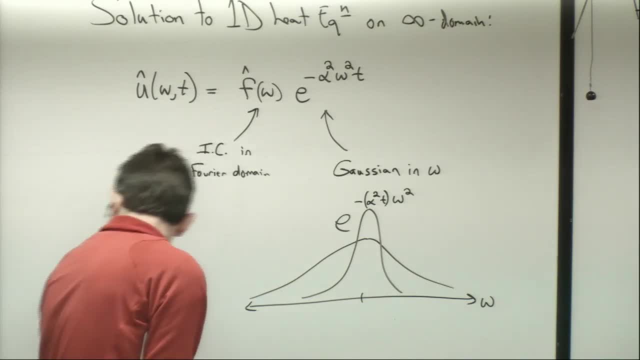 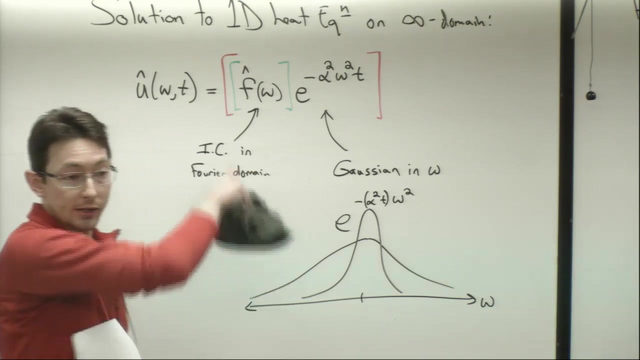 before we even inverse, transform, OK, so I like to use colors here. I'm going to say that this is the red part of the equation and this is the green part of the equation, And what we're going to do now is we're going to inverse. 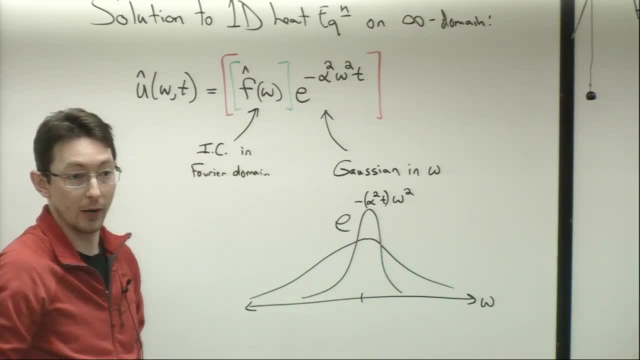 Fourier, transform this to get our solution in space. We have our solution in frequency. Let's inverse Fourier, transform it and get a solution in space. OK, And in the next lecture, what I think we can do this is either for the next lecture or for homework. four: 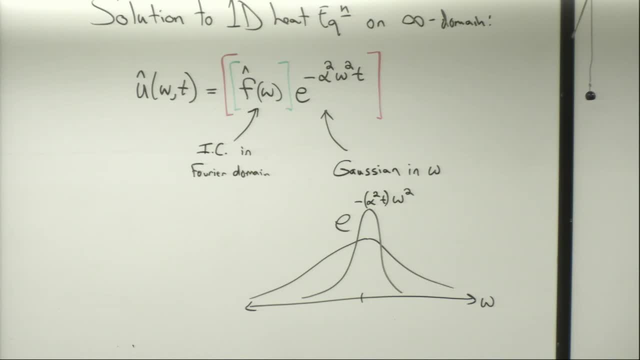 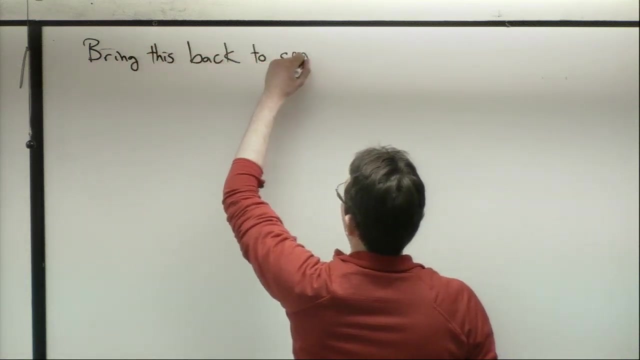 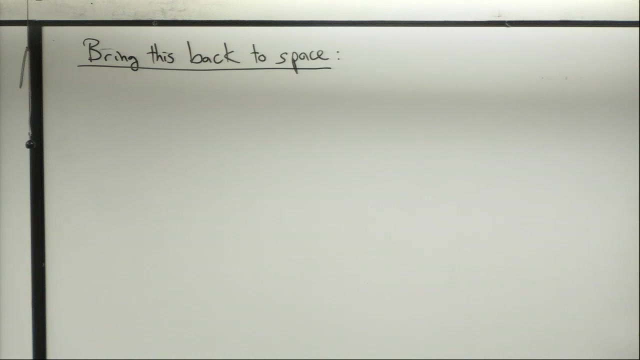 is we're actually going to start plotting solutions of this for different initial condition distributions because it looks neat. OK, so we want to go back to space where we live. OK, so to bring this back to space, we inverse, Fourier, transform. OK, there's three nasty integral steps. 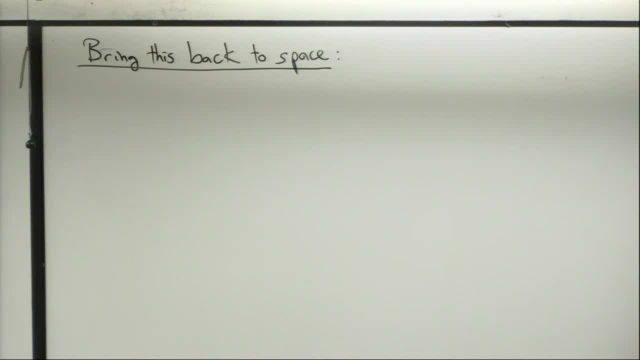 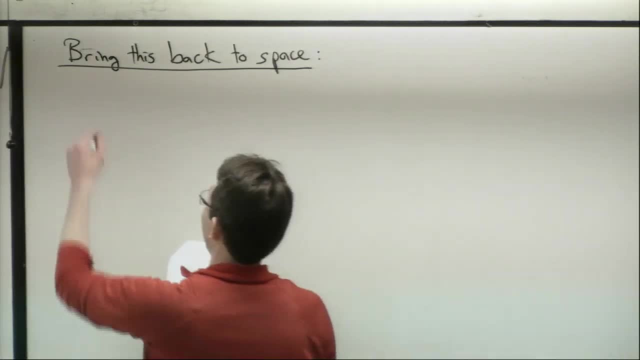 but they're not that nasty and I'm going to take the worst part and just tell you what the answer is. This was the worst integral I've ever done and I'm not going to make you do it. So my temperature as a function of spatial variable x and time t. is given by my inverse Fourier transform of the integral of x. So I'm going to take the worst part and just tell you what the answer is. So I'm going to take the worst part and just tell you what the answer is. So I'm going to take the worst part and just tell you what the answer is. 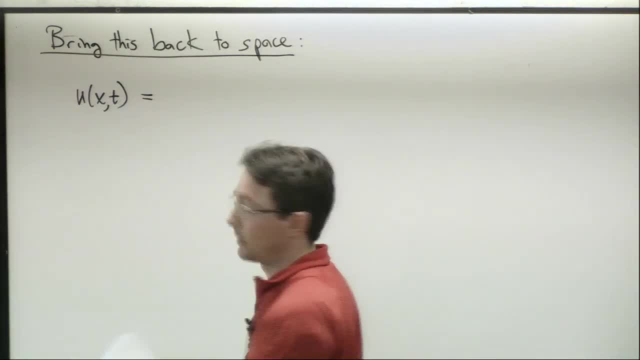 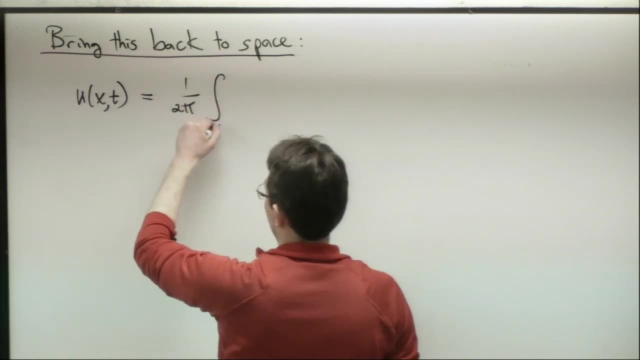 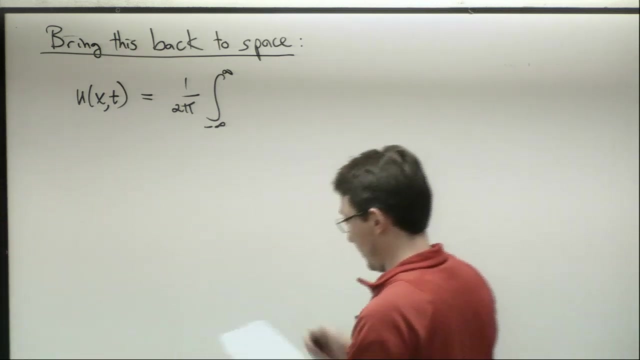 of the frequency domain solution. So what's my inverse Fourier transform- Maybe you can just read it to me: 1 over 2 pi minus integral of infinity to infinity of this nice expression here. whatever, let's say that there's some red bracket stuff. 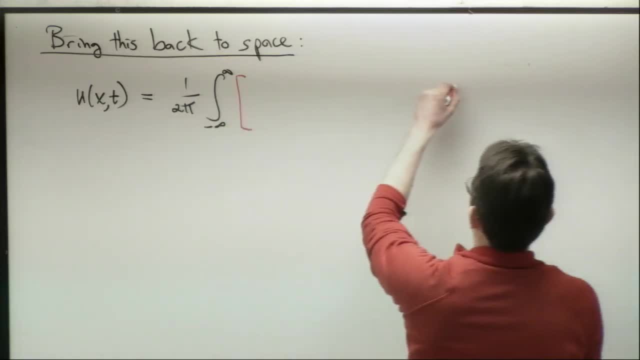 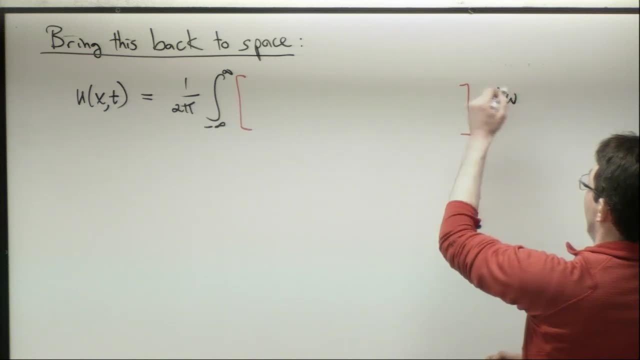 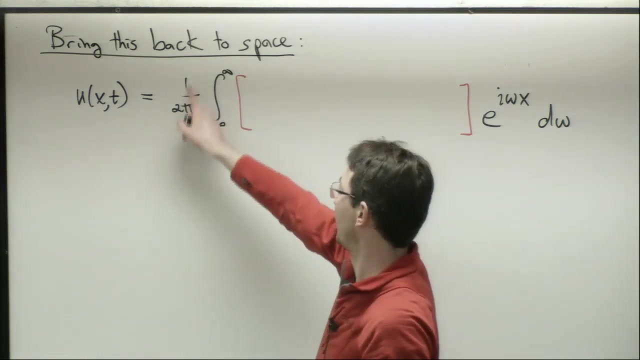 my function. big red bracket of stuff times e to the positive, I, omega, x, d, omega Sound right? That's the inverse Fourier transform. I have a 1 over 2 pi here because you need it to be if you want the inverse to be the identity. 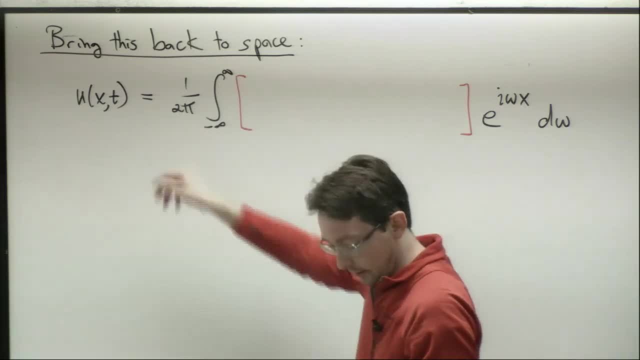 the inverse, composed with the Fourier transform, should be the identity. so I need this 2 pi here. Some people put a 1 over square root of 2 pi on each of the Fourier transforms, but I like this one better. It's easier. 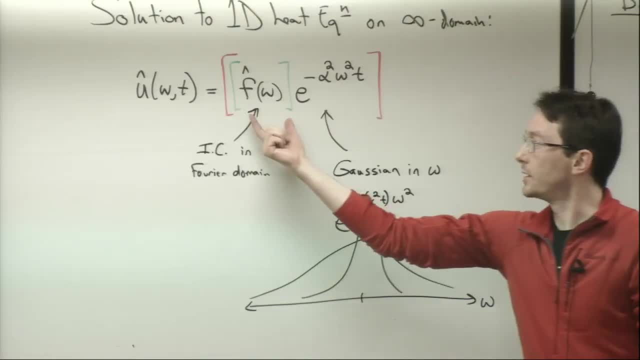 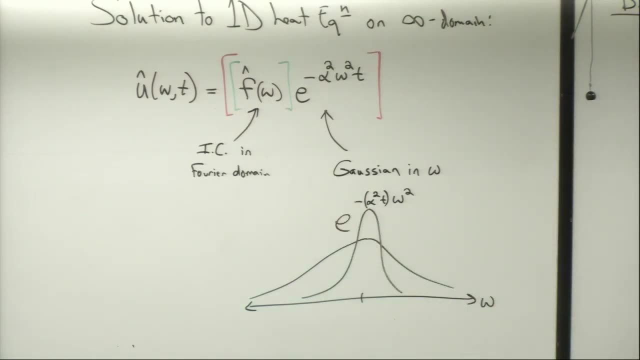 Okay, so the stuff inside the red integral. I'm going to expand this green part out as another integral. I need to do that to solve this. Okay, that's why I wrote it in colors like this. So the green part: what's f? hat? 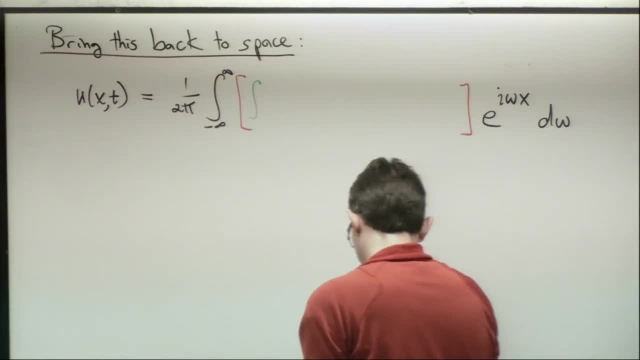 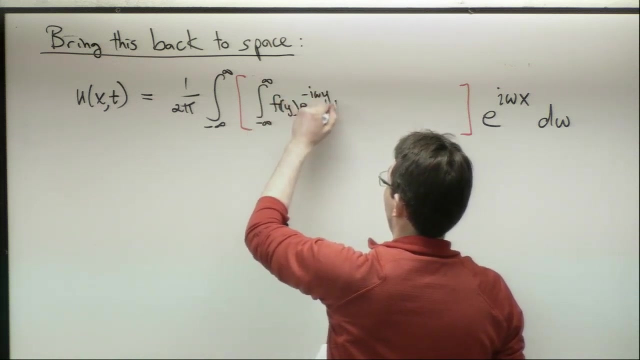 It's the integral. okay, it's the integral from minus infinity to infinity, of f of x. I'm going to use a dummy variable. I'm going to call it f of y. e to the minus i, omega, y, dy, That's f hat. 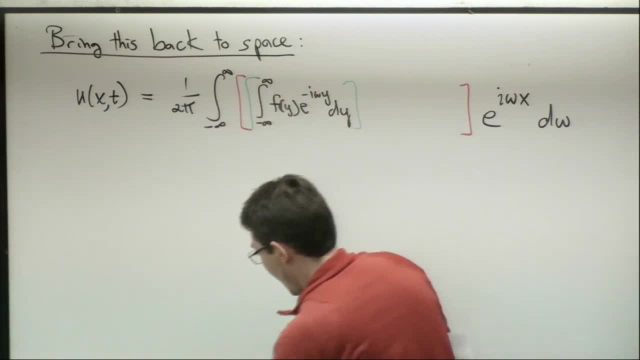 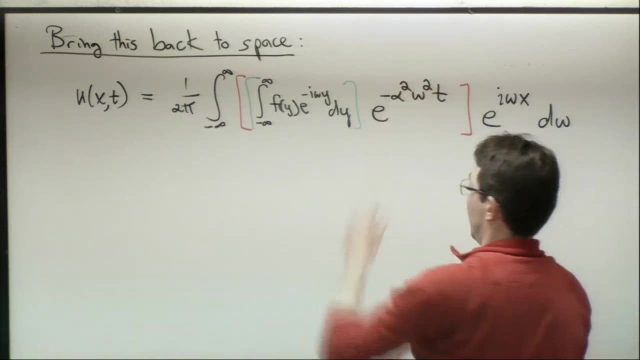 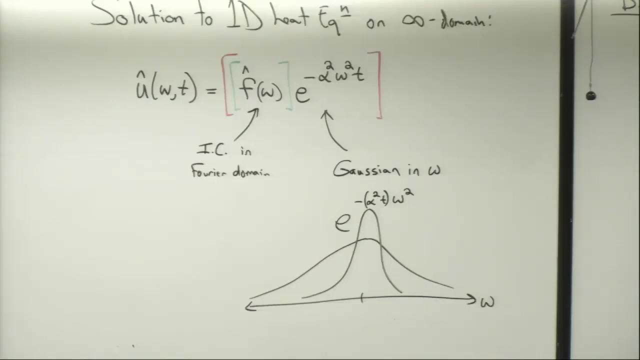 Okay, that's my green piece. And then the other piece is e to the minus alpha squared, omega squared t. Okay, this isn't super complicated right? I'm just taking the inverse, Fourier transform of that expression in the red brackets and I'm expanding out f of y. 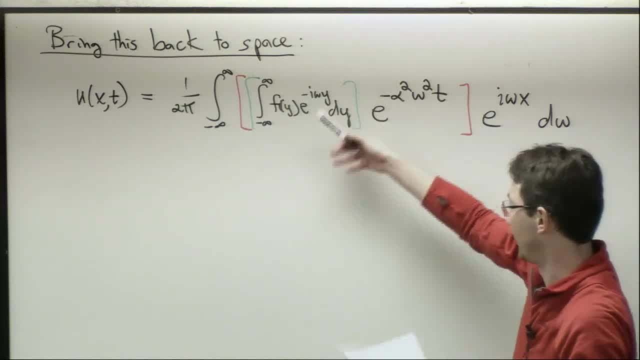 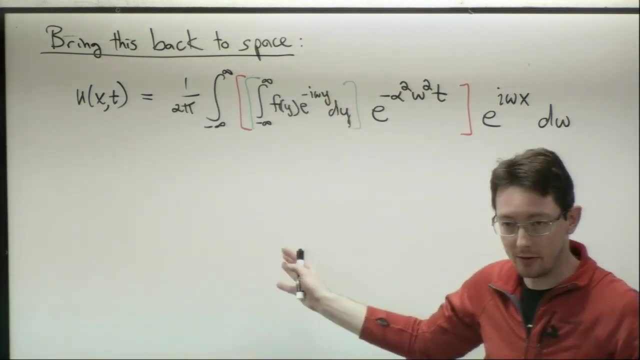 I'm expanding out f hat so that it's written in terms of, so that it's explicit what I'm talking about here, And I'm using a dummy variable, y, because it would be super confusing if I used x. Okay, now, what I'm going to do is the following: 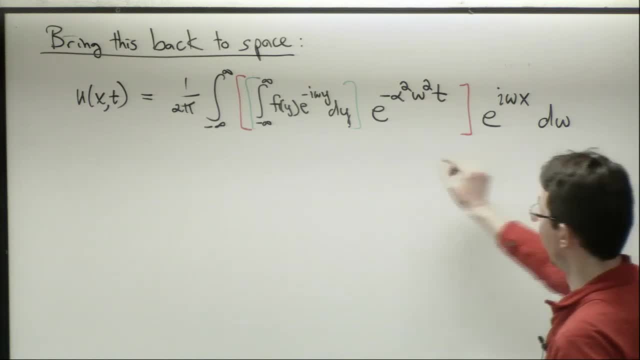 Neither of these terms has a y in them, And so I can take this dy and I can bring it out farther, So I can bring this entire thing into a big double integral And I can group different exponential terms. So I can take e to the i, omega x minus y. 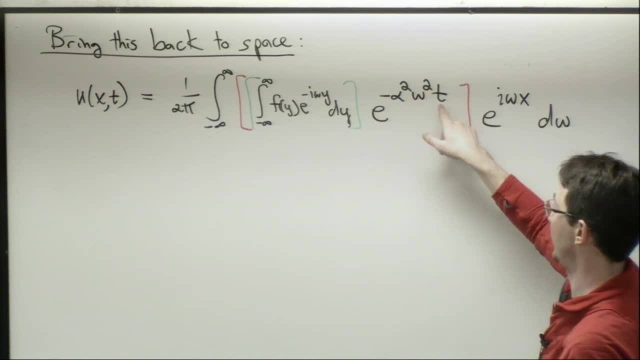 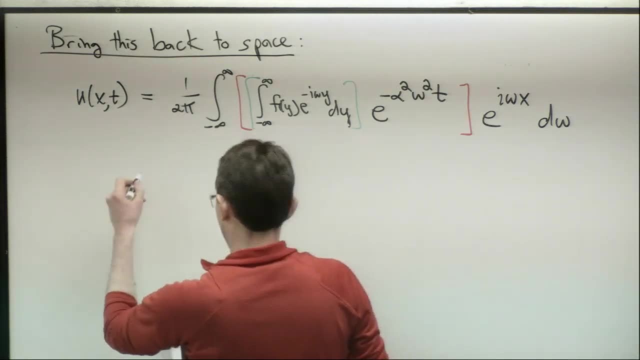 times e to the minus alpha squared, omega squared, t times f of y. I'm just regrouping the insides and I'm making a double integral. So this equals one over two pi double integral, both of them from minus infinity to infinity. 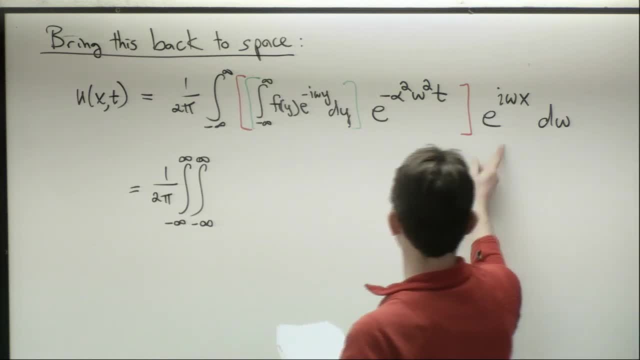 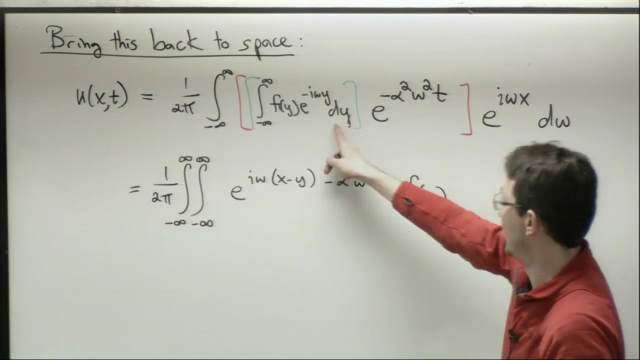 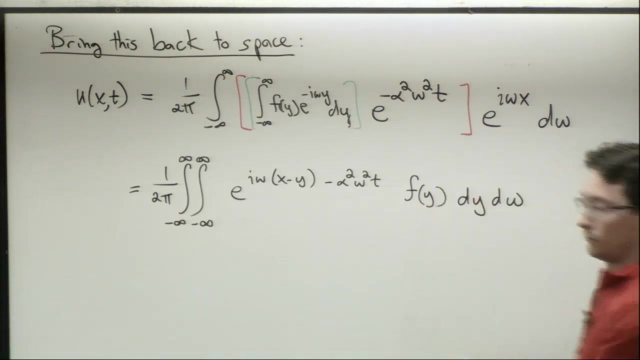 Of e to the i omega x minus y minus alpha squared omega squared t times f of y And it's dy d omega. Stop me at any point if this becomes confusing or weird or if I do something wrong, But it's pretty standard. 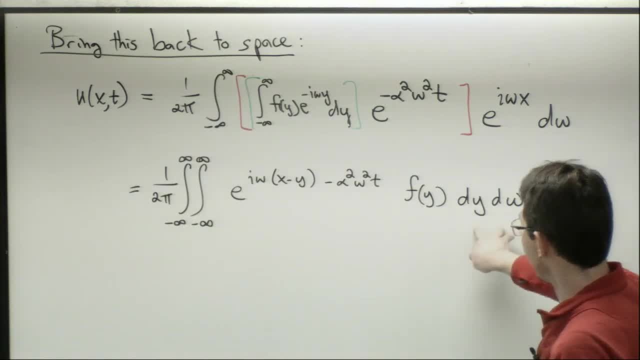 I'm just rearranging stuff, Okay. Now what's nice about this double integral is I can switch the order of integration. I can integrate omega first and then y, It doesn't matter, And that's what I'm going to do. So I'm going to bring this. 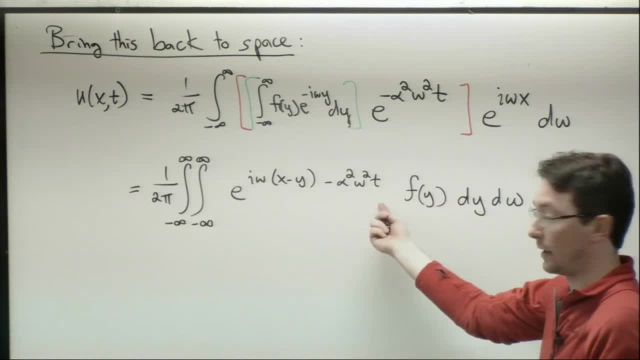 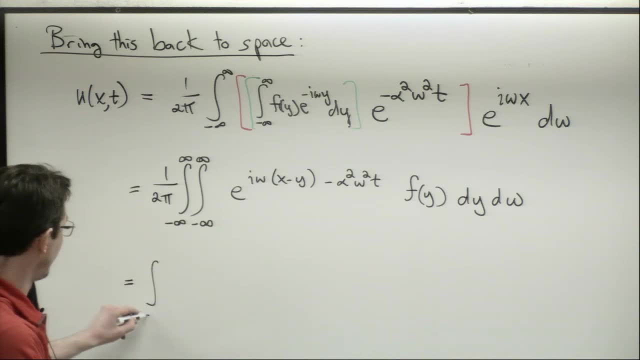 And this function of y doesn't have an omega in it, So I can bring d omega in here And what I'm going to get is the following: This is equal to the integral function of y, The integral from minus infinity to infinity, of one over two pi. integral minus infinity to infinity. 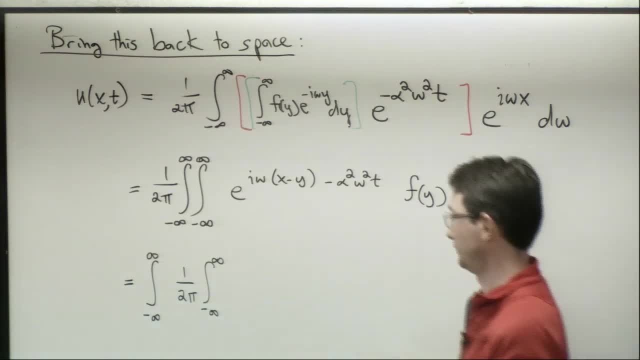 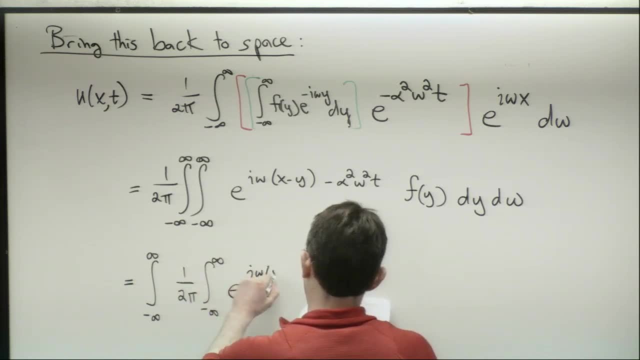 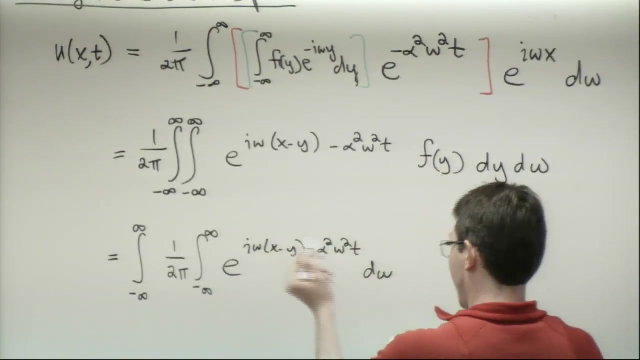 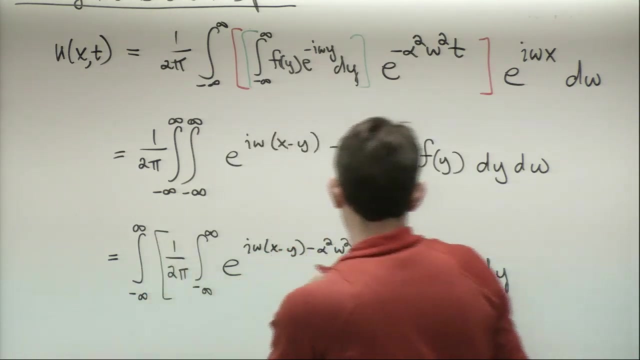 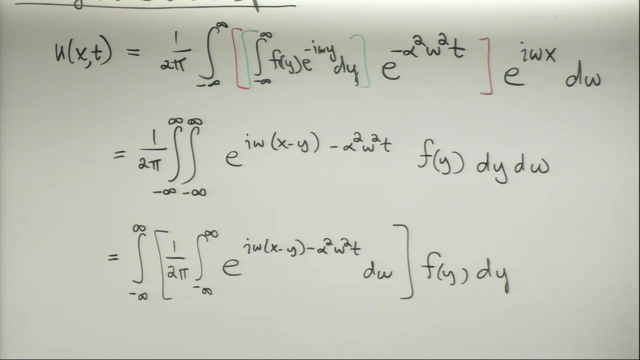 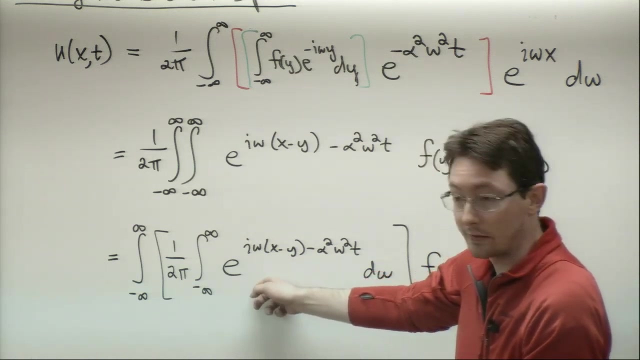 of this expression: d omega E to the i omega x minus y, minus alpha squared omega squared t d omega times f of y, dy. This is all simple integration tricks, okay, But now this integral is starting to look, to me at least, a lot like a inverse Fourier transform. 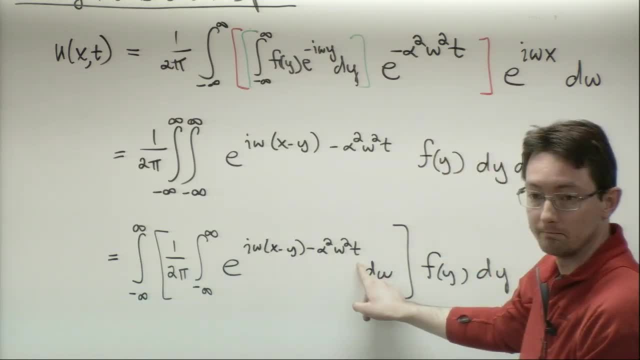 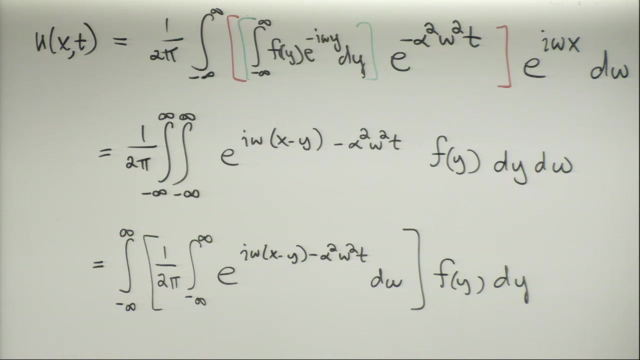 of e to the minus alpha, omega squared t. So let's zoom into this integral for a little while. So this is a little tricky. We have to zoom into this inside integral to figure out what it means. Okay, so we have to figure out what this expression is. 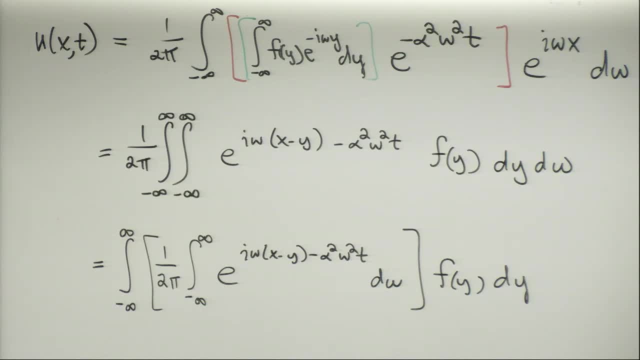 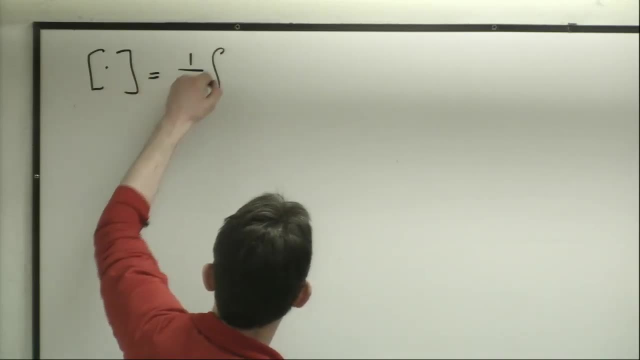 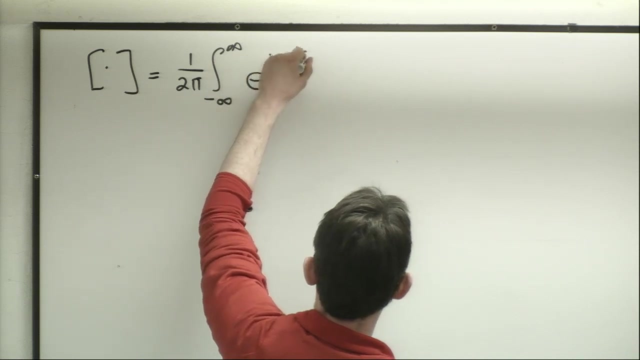 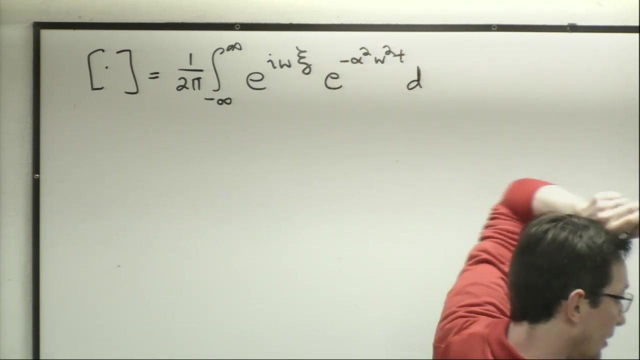 So we have. Okay, so the stuff inside the brackets is equal to the 1 over 2 pi integral minus infinity t to infinity of e to the i omega xi times e to the minus alpha squared omega squared t d omega, where I've introduced another dummy variable. 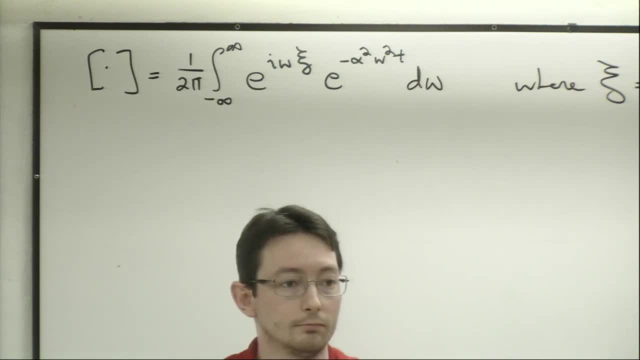 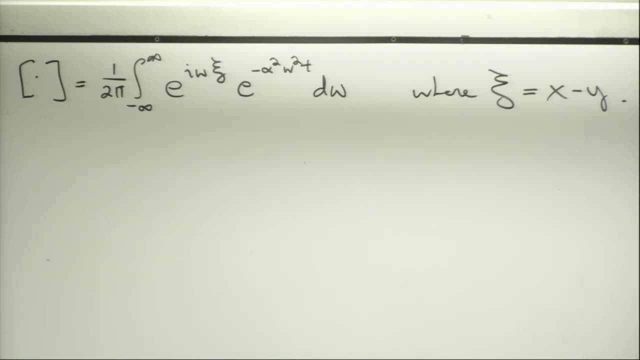 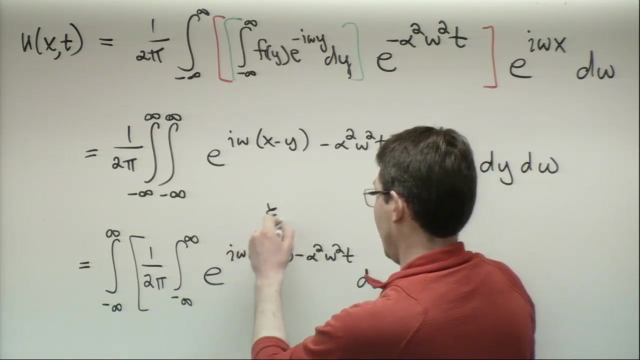 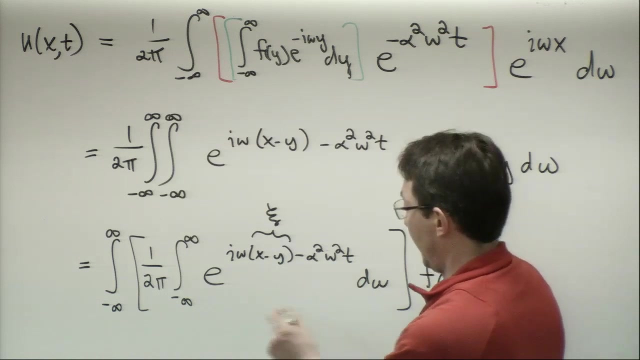 xi equals x minus y. This inside integral right here is: e to the i omega times, e to the minus alpha squared omega squared t Right, If I multiply two exponentials, then the exponential parts just add. So that's what this inside bracket is. 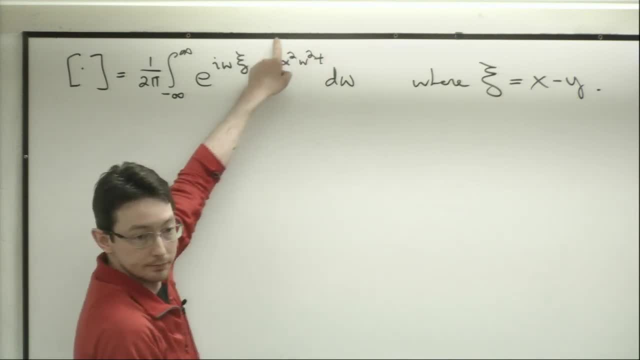 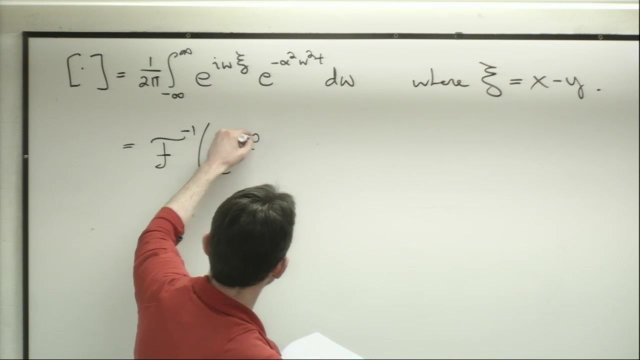 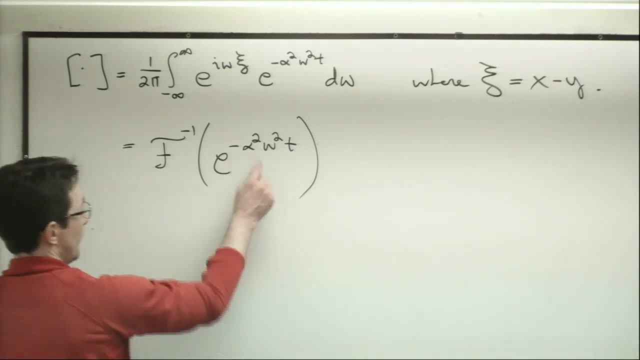 And this is exactly the inverse Fourier transform of this thing. I'm just, in terms of this dummy, variable xi. Okay, So this is equal to f, inverse of e, to the minus alpha squared omega squared t. Remember what does this function look like in omega? 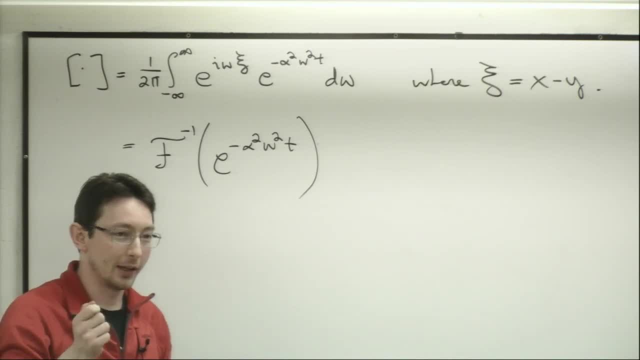 Gaussian. right, This is a Gaussian function. Now, the really, really nasty integral that I don't want you to have to do, that I try to forget about, is that this inverse Fourier transform, this integral here, is also a Gaussian, So this is an extremely important fact. 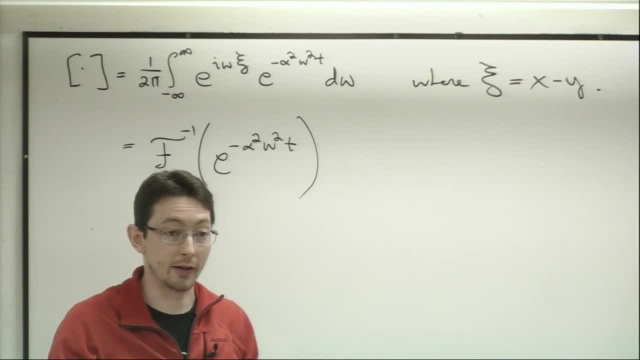 that I don't want you to have to verify. The Fourier transform of a Gaussian is another Gaussian And the inverse Fourier transform of a Gaussian is another Gaussian. This is an extremely, extremely, extremely useful property. This is one of the most important facts. 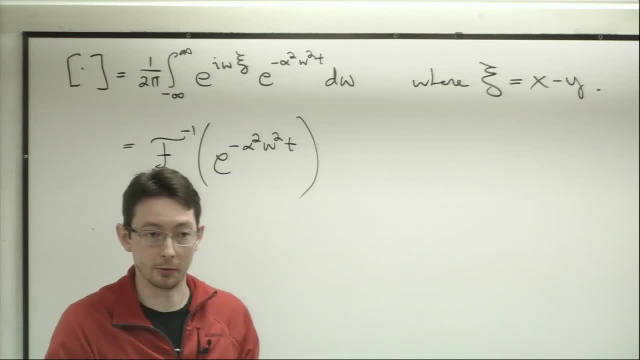 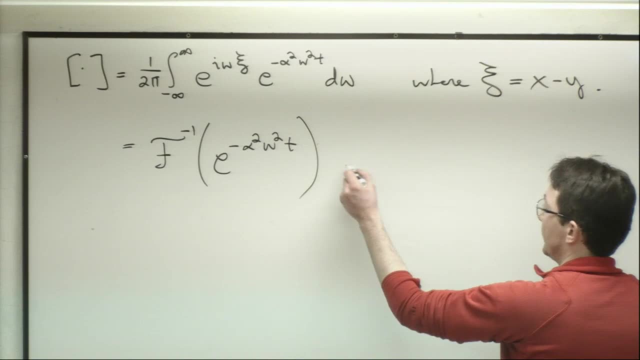 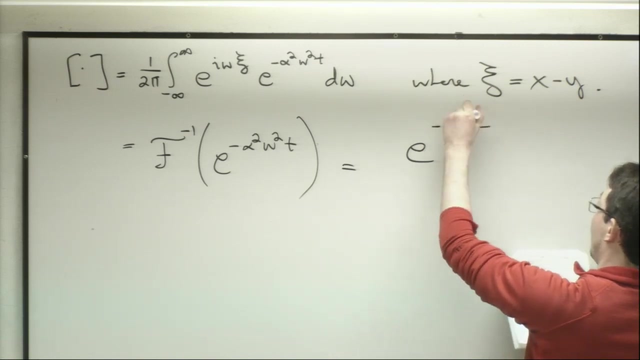 about Fourier transforms. probably the second most important after the derivative property, is the fact that Fourier transform of a Gaussian maps to another Gaussian. Okay, so this equals another Gaussian, And I'm just going to tell you what it equals. It equals e to the minus c squared divided. 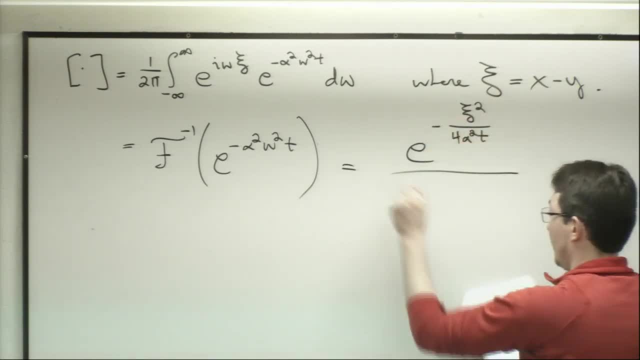 by 4 alpha squared time. this whole exponential divided by- I don't know, I don't know. It's divided by 2 alpha square root of pi times time. Okay, This 2 alpha square root of pi times time is my variance. 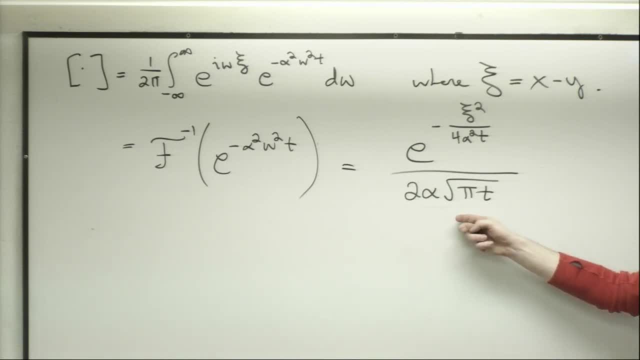 Variance may be the standard deviation. It's one of those. I think it's the standard deviation and this is the variance, And that means that my variance and my standard deviation grow as t grows. This thing spreads out as t increases. 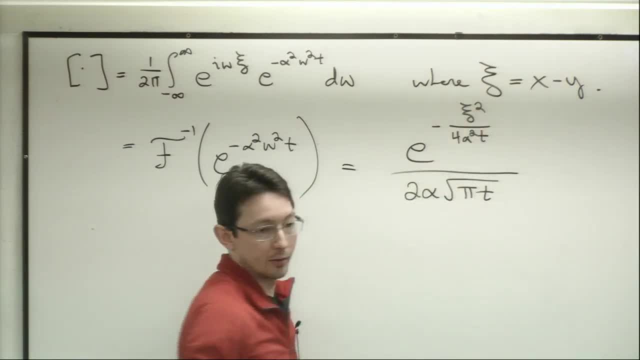 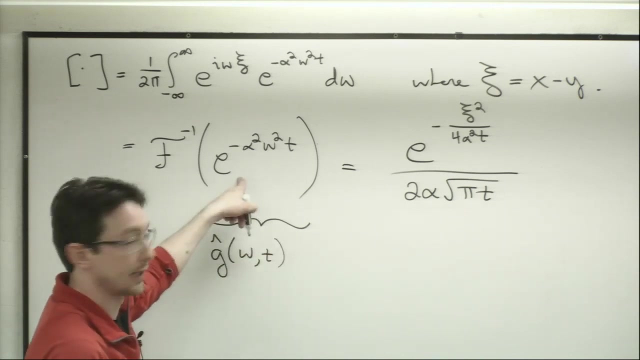 And remember this is a function of space. now, This is x minus my dummy variable y. Okay, so I'm going to call this thing in here. I'm going to call this g hat of omega in time. I'm using g because it's a Gaussian. 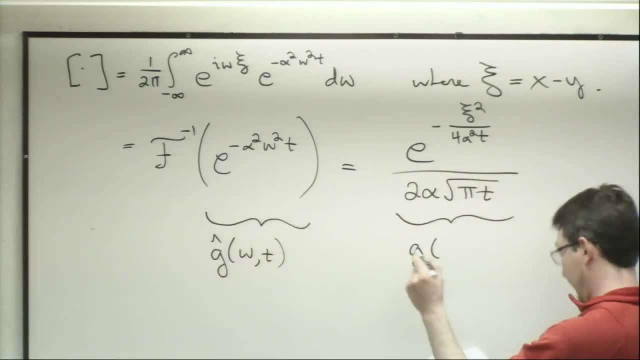 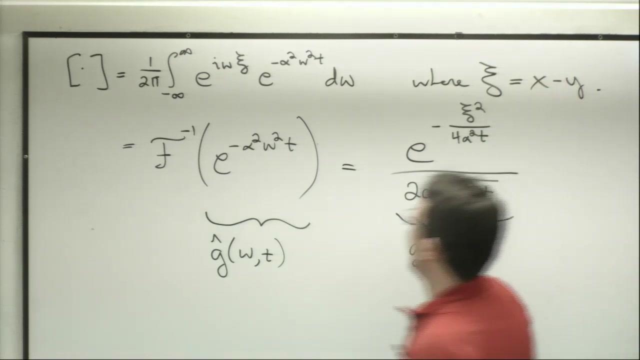 And I'm going to call this g of xi. in time, Xi is kind of It's a spatial-like variable, It's in space, but it's x minus y. Okay, does the basic idea make sense? I take the Fourier transform or the inverse Fourier transform. 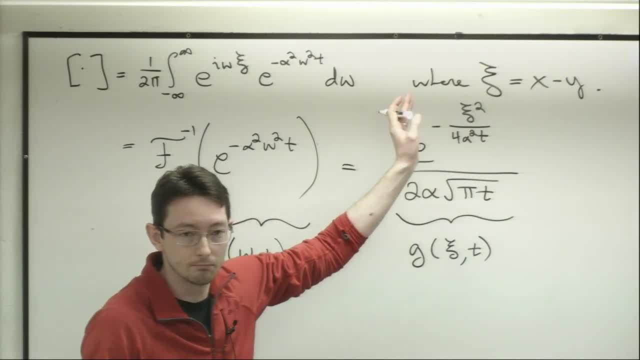 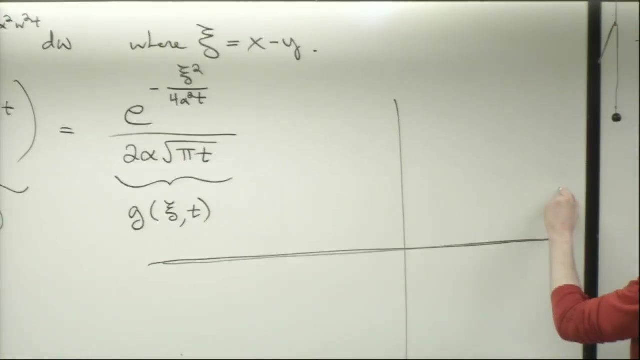 of a Gaussian, I get another Gaussian, but it has some weird variance. And to compute this integral, to compute this integral here we have in the complex plane, we're trying to compute this integral, It turns out what you would do is you would create. 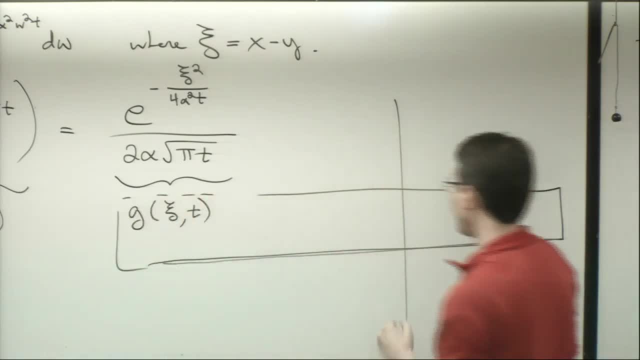 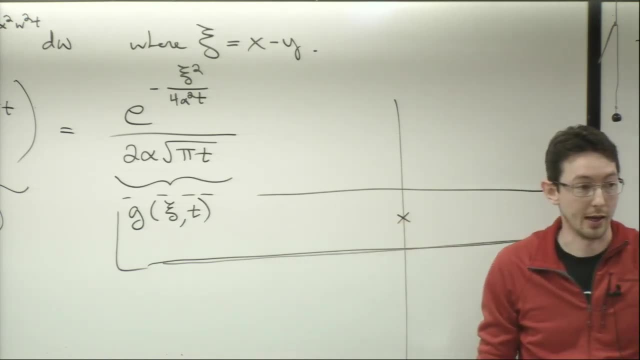 right A weird-looking box integral and you would have some residue, some poles here and you would use all of the Cauchy integral formula stuff that we learned in the first part of the class So you actually can solve this integral using complex. 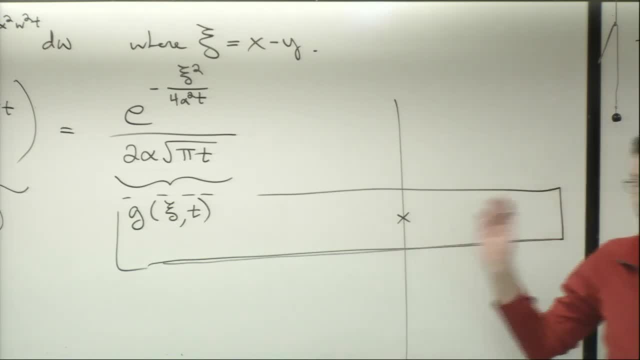 integration theory, but it's horrific And you can look it up on Google. okay, Inverse Fourier transform of a Gaussian- easy. okay, It might be a good thing to look at someday. Okay, good, Now we know what this term is. 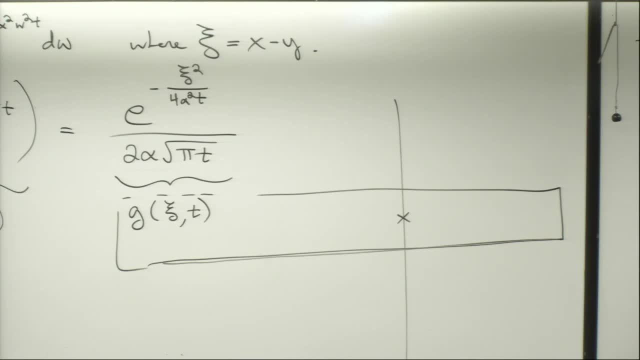 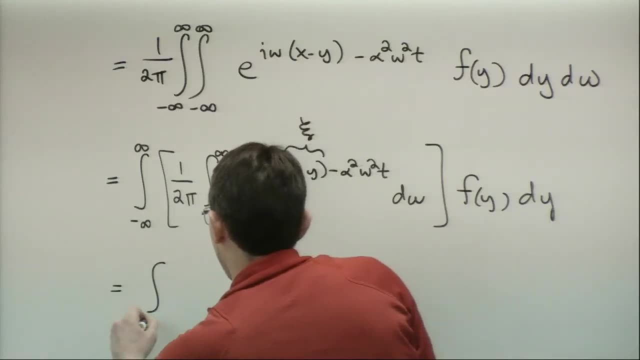 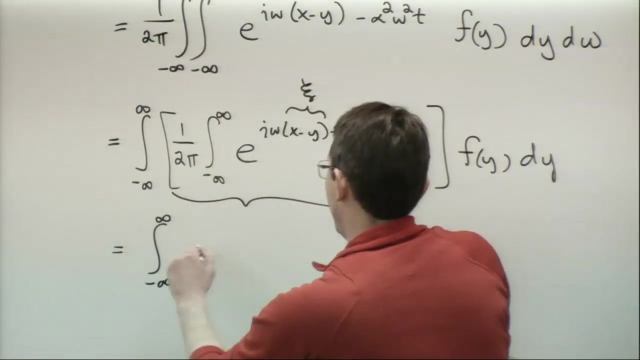 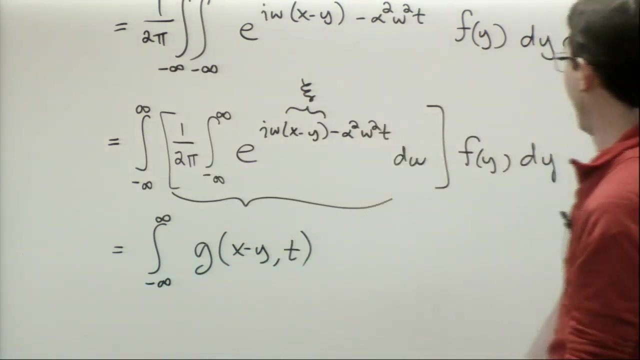 This inner term here in the brackets is what It's: the inverse Fourier transform of my Gaussian. This is just equal to g of c comma t. So I have the minus integral from negative infinity to infinity of g of x minus y and time times, f of y, dy. 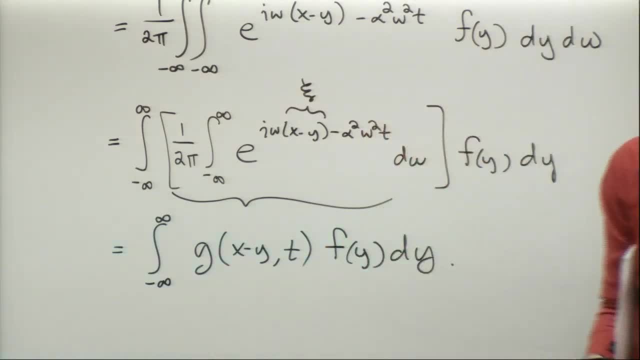 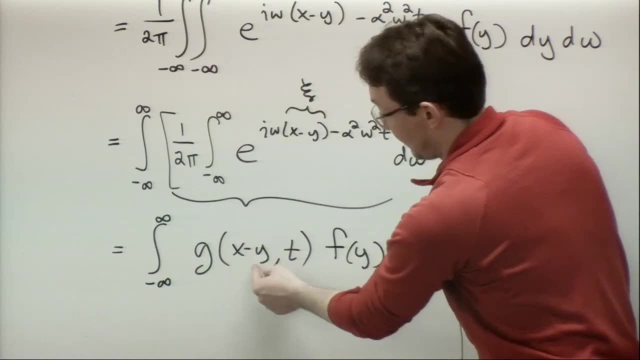 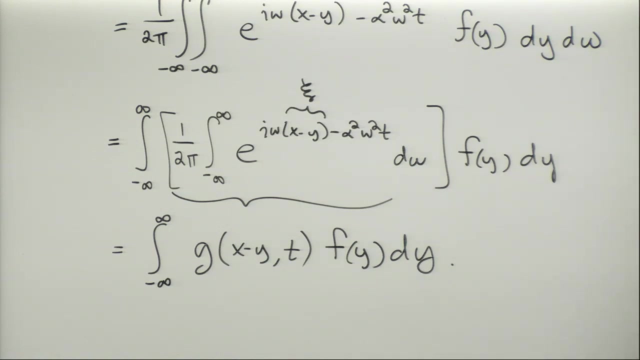 And all of a sudden it looks much, much simpler. Okay, so this dummy variable c is really x minus y, And so I have my Gaussian, that funky Gaussian of x minus y comma t. Okay, what does this integral look like? 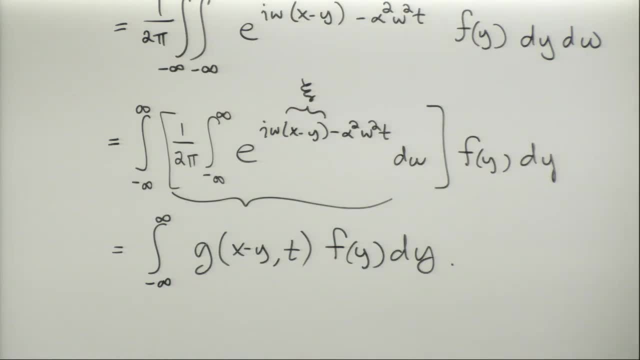 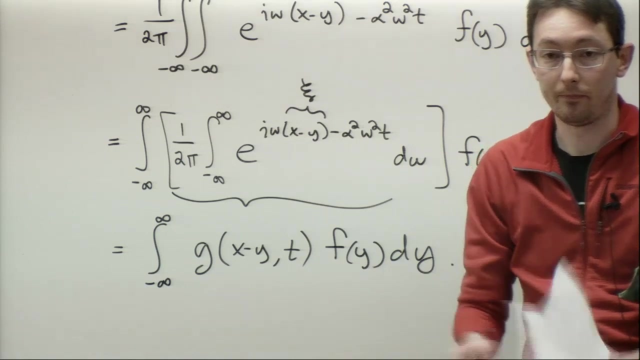 What does this integral mean? Okay, it does look like an inner product, but that's not exactly what I'm going for. It does look a lot like an inner product, But this x minus y means that this is a convolution integral. Okay, so how many of you remember convolution integrals? 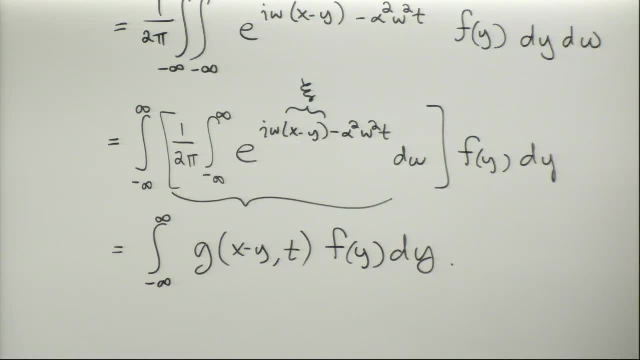 or have seen them before. Okay, how many have not seen convolution integrals before? It's okay, Okay, good. So for now, I'm just going to tell you that this is called a convolution integral. This integral is a convolution integral. 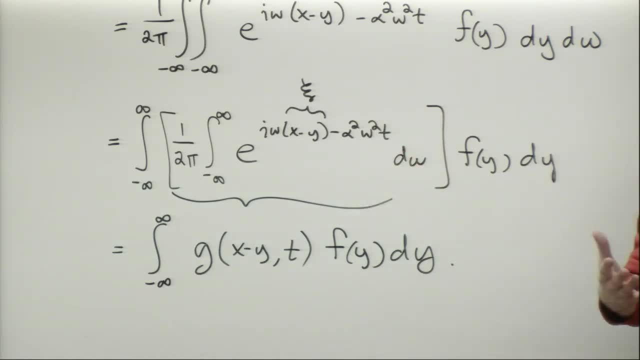 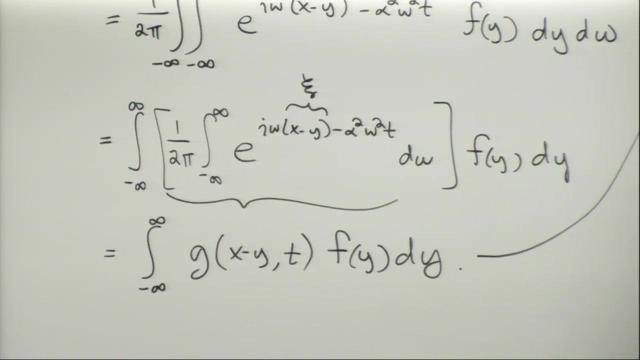 And when we do Laplace transforms, I'm going to really give you some intuition for what the convolution means physically. It's got very deep physical meaning and I'll have time to tell you that a little bit next week. So this equals. the notation for this is g, star f. 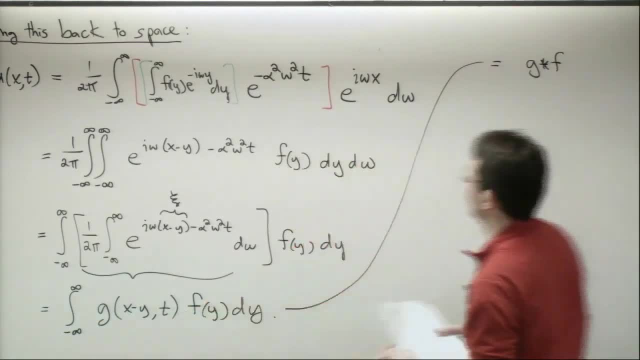 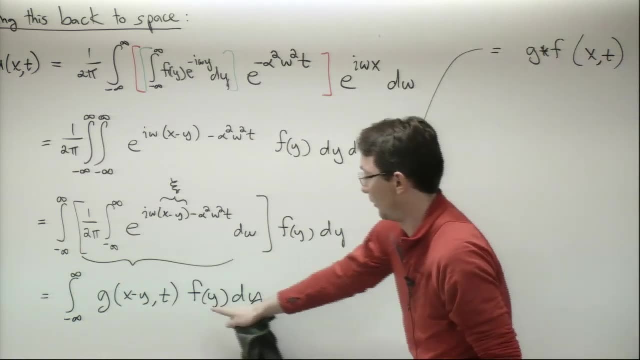 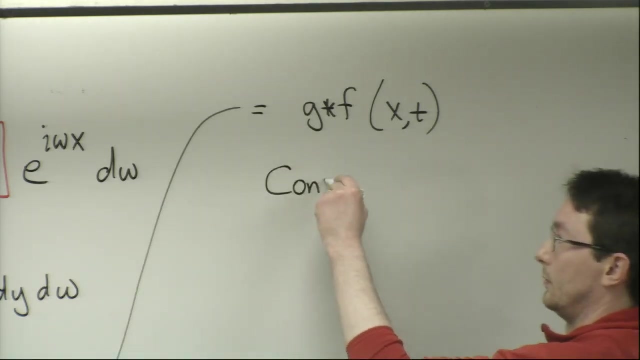 That's what this we call. this integral is g, star f. This is just a symbol we use And this is a function of x and t, because I'm going to integrate out my y variable. Okay, and this is called convolution. 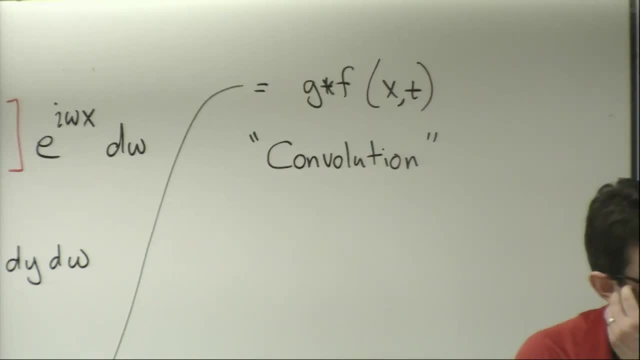 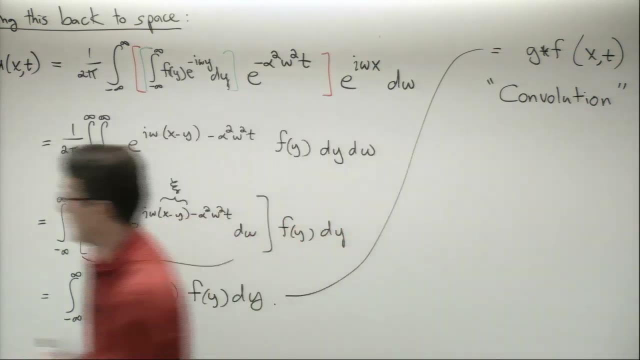 Okay, so we're going to very shortly, at the beginning of next week, we're going to start building an intuition for what this convolution means physically, And I'm going to start showing you what it means right now. It basically means that all of my function f 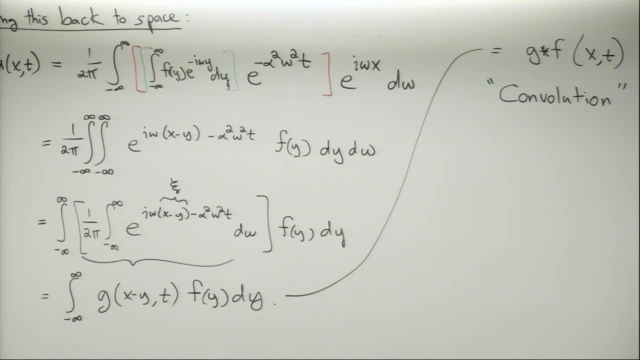 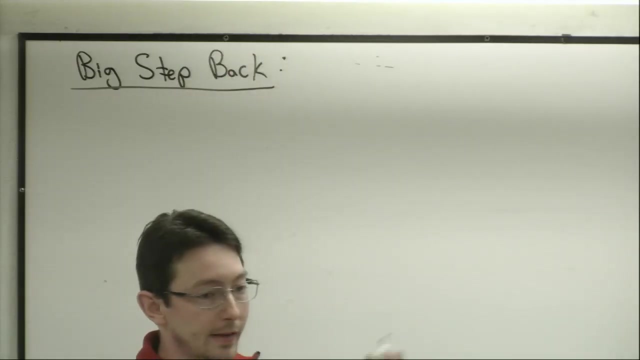 is going to spread out because it's being multiplied by a Gaussian and integrated, So that's going to be our solution. Okay, good. So now we're going to take a big step back and we're going to think about, physically, what we've learned about the system. 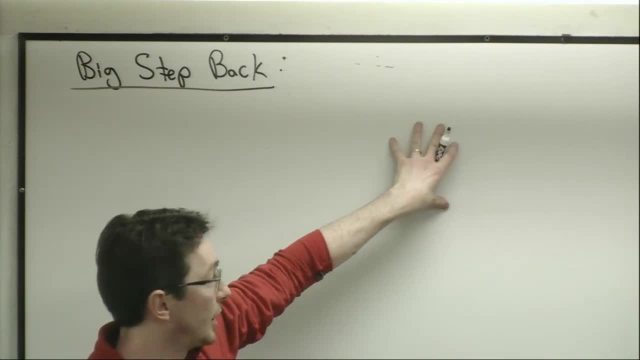 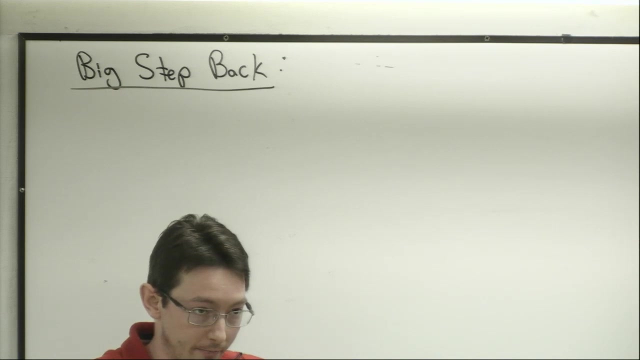 Okay. so in the frequency domain, we wrote down our solution: u hat omega t And we saw that it was our initial condition: times time. okay, and what that means is that all of my frequencies, all of my frequency content of my initial conditions were being damped out. they were dying out, spreading out in time and they 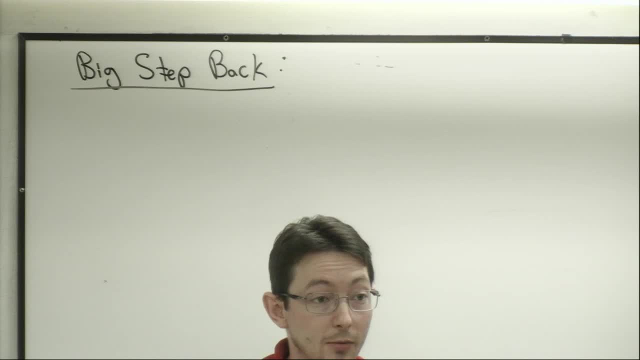 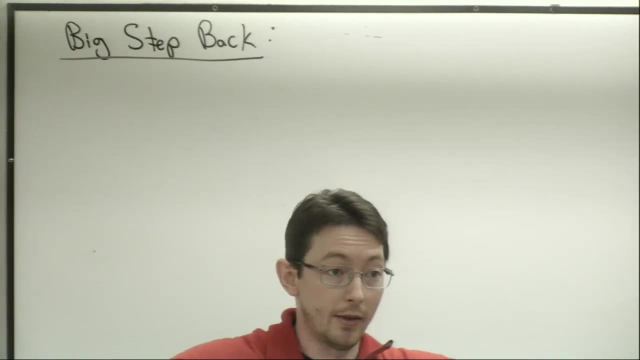 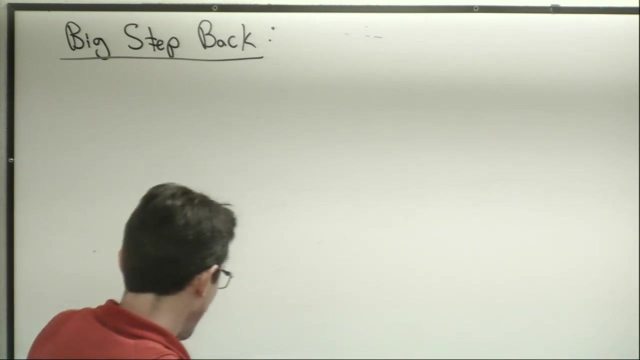 eventually would spread out to, uh, to zero, because that gaussian would eventually become completely flat. one of the important properties of a gaussian is that it always has unit area underneath the curve, and so if i have infinitely long variance, then it's infinitely shallow, okay, um, so what i 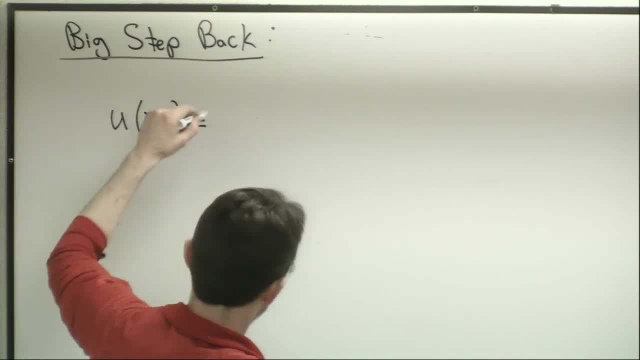 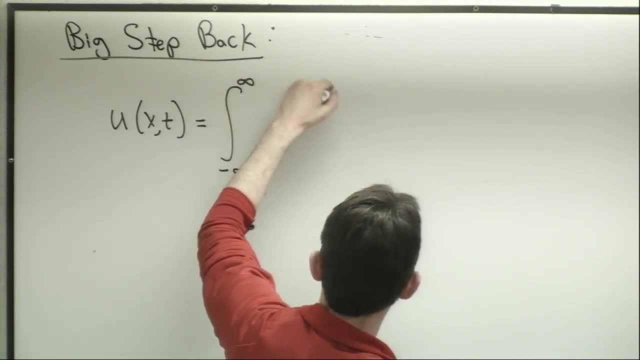 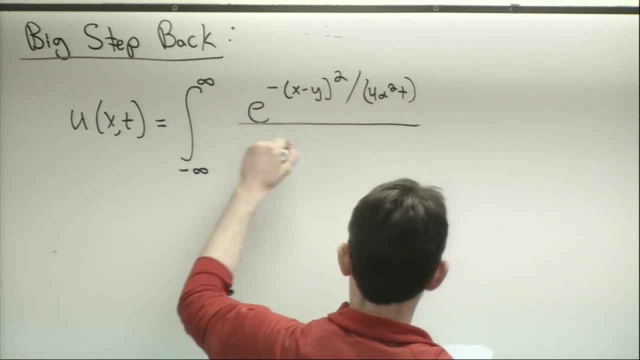 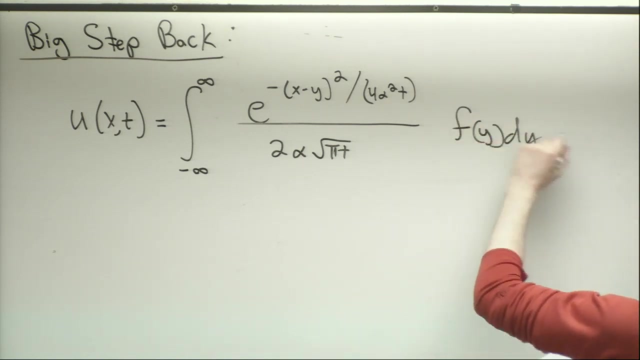 have is my u of x comma t equals this big nasty convolution integral, integral, minus infinity to infinity, of e to the minus x, minus y, squared, divided by some stuff for alpha squared t, divided by two alpha root pi t. okay, so this is my big convolution integral. 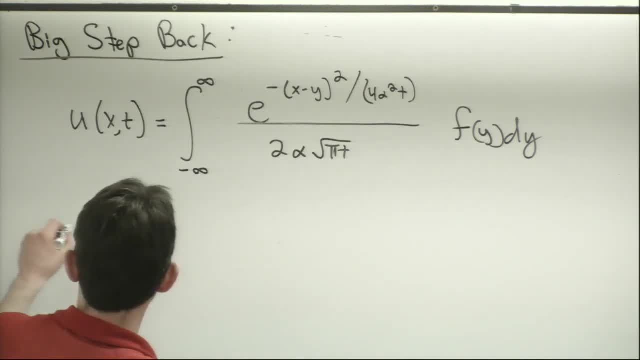 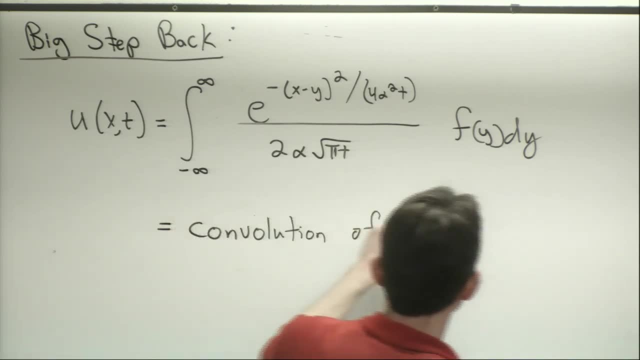 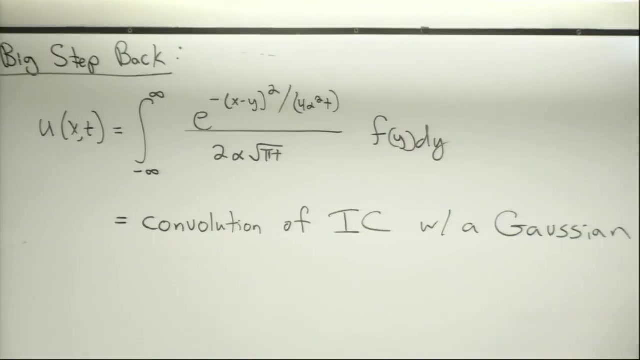 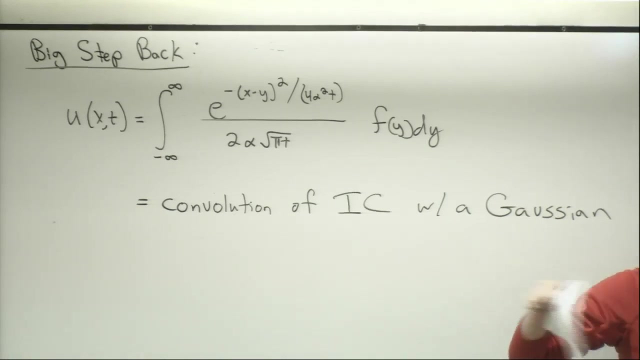 and so u of x and t equals convolution of initial conditions with a gaussian. so, in words, this is what the partial differential equation is doing: we're convolving our initial conditions with a gaussian. we're spreading out all of the variances and differences in our initial 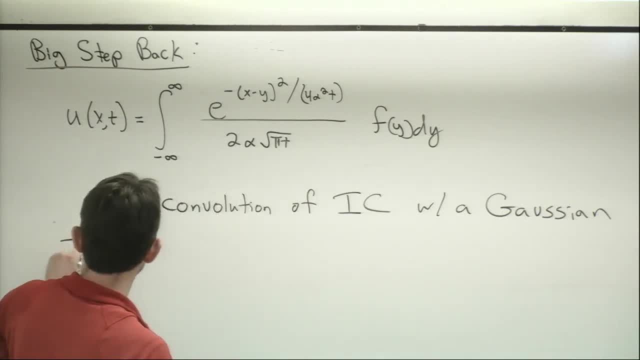 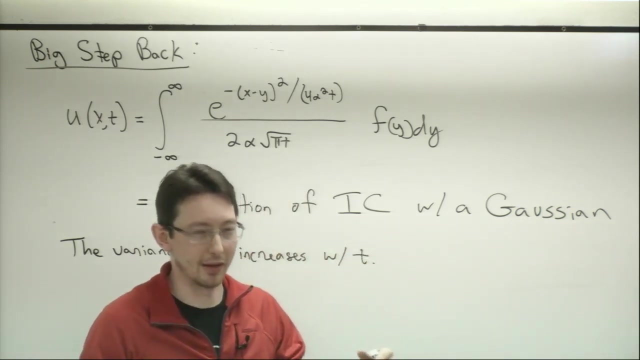 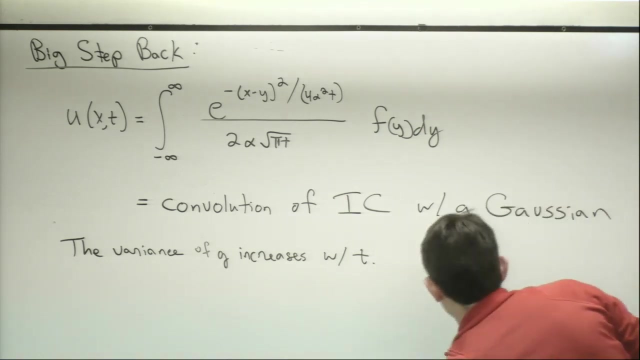 conditions and we're convolving our initial conditions with a gaussian and the variance of our gaussian g. the variance of g increases with time or with the square root of time. i think it's with time. the standard deviation increases with the square root of time and so if i had imagine i had an initial temperature distribution, this is x. now we're in space. 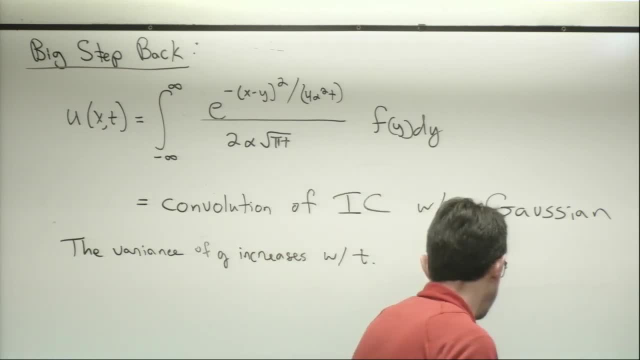 and let's say that this is x and we're in space. x equals zero. So if I have an initial temperature distribution which is like a spike in temperature at zero, you can think of this as either a really, really big temperature in a small 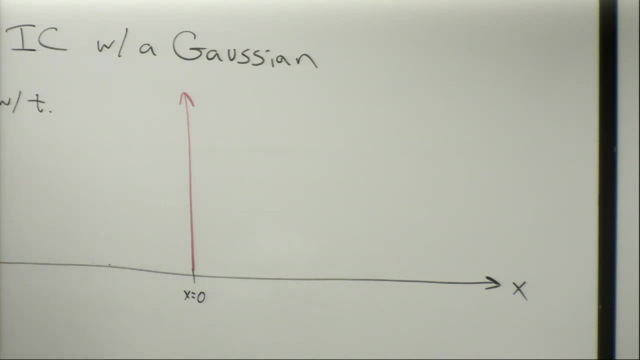 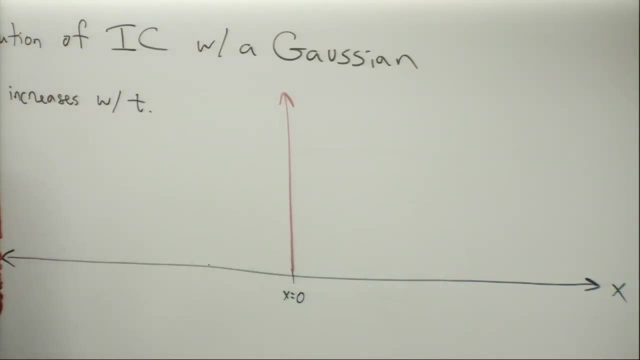 window, or you can even think of it as a delta function if you like. And the way I think about this. let's say I have my steel rod and I just apply a blowtorch to this location. It's got a really big spike in temperature, big blowtorch spike in temperature, and then 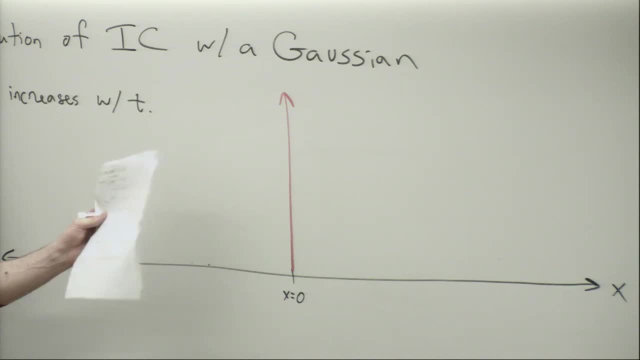 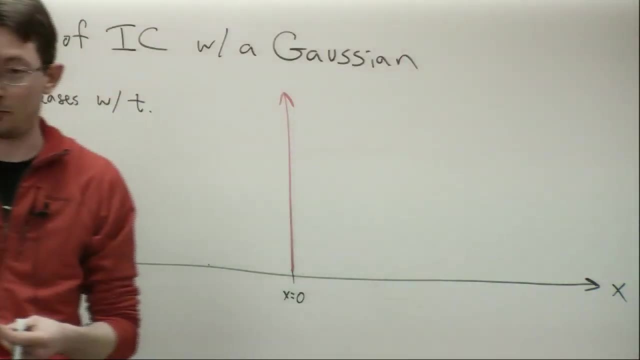 I turn the blowtorch off and let it go. What's going to happen? It's going to spread out, okay, And I wish I had a blue pen. I don't have a blue pen. I have a blue pen at my office. 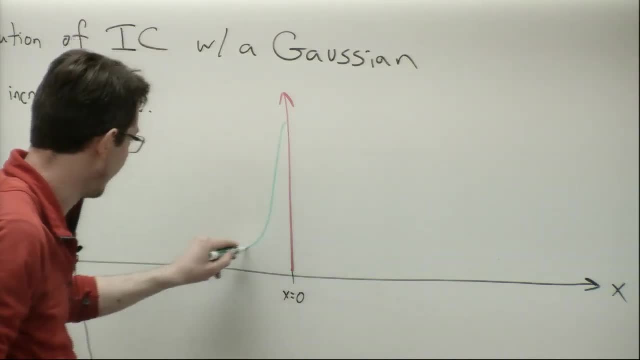 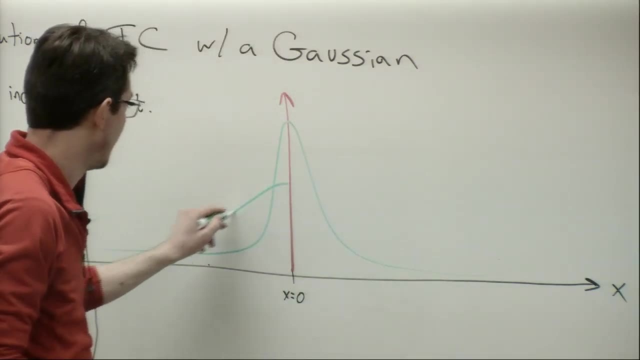 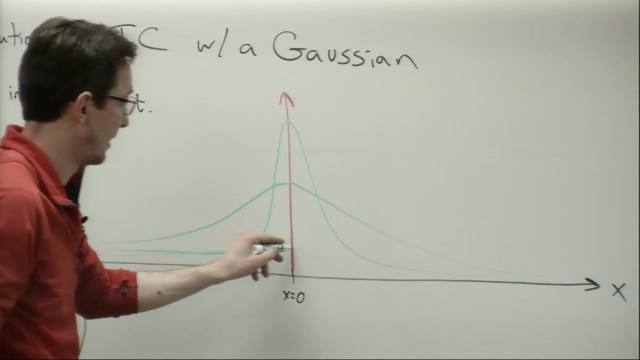 but I have a green pen here, And so what happens at very short times is that this immediately spreads out, and as time increases it becomes more and more spread out, because my Gaussian has higher and higher variance, and eventually this becomes kind of infinitely. 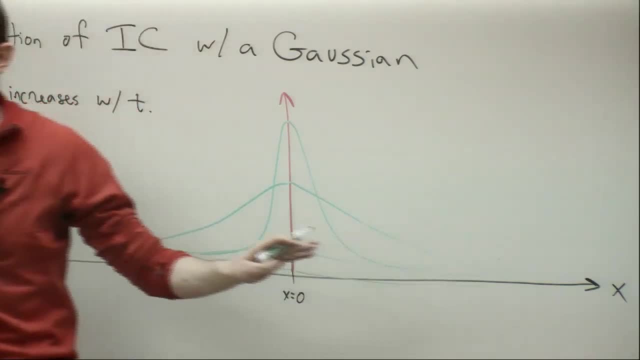 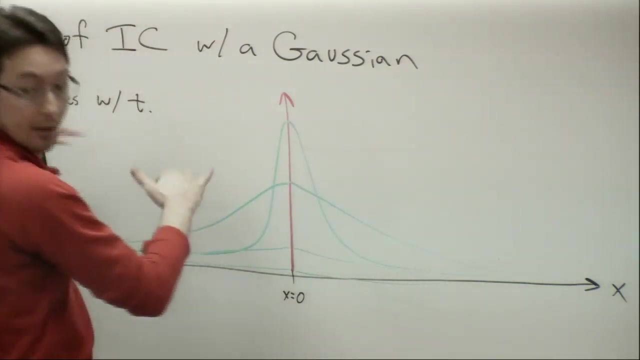 infinitely shallow and there's zero temperature everywhere. All of the thermal energy gets distributed across all of infinity. So this is physically what we mean by convolving our initial condition with a Gaussian. It's every initial temperature disruption gets smoothed out eventually and eventually goes to zero. And when we start plotting this solution, 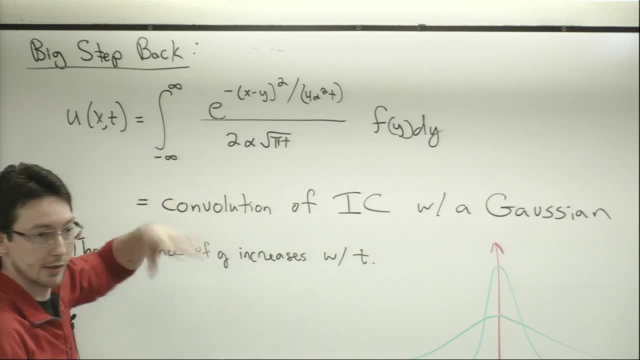 we're going to see very clearly that that's exactly what happens in MATLAB. This is not just some, you know, it's not just words. I'm saying: This is actually what the equations are saying. Okay, that's basically what I have. Are there any questions? 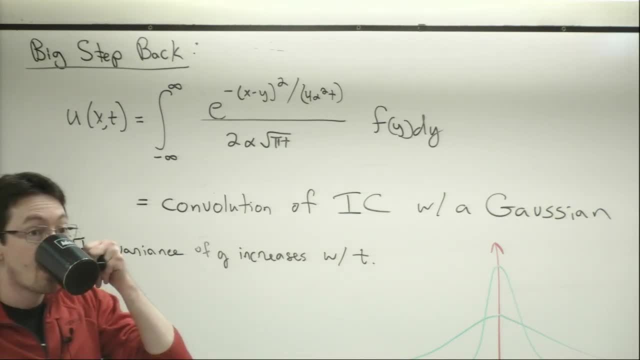 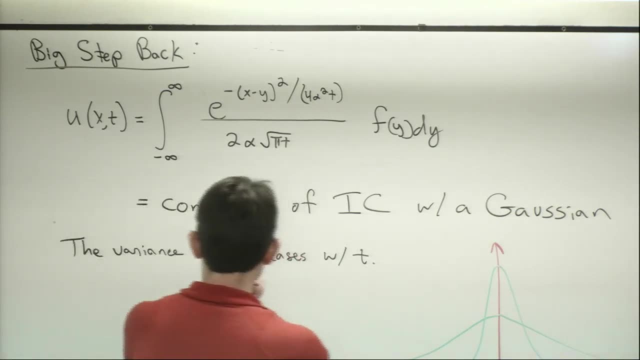 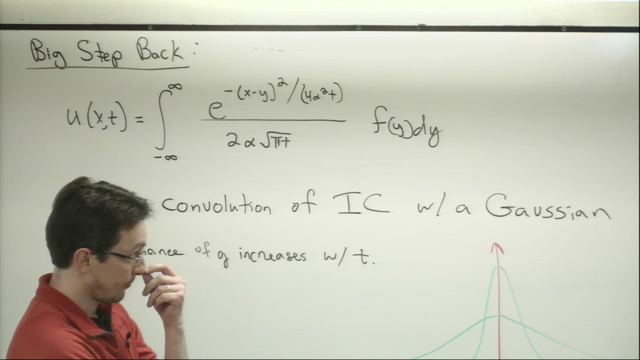 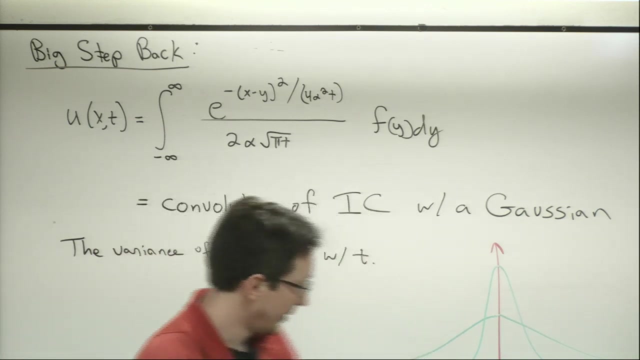 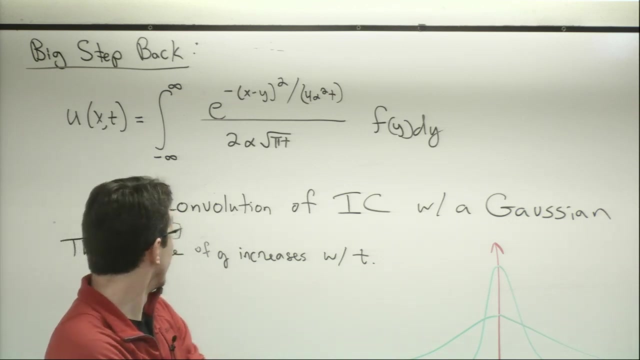 Yeah. So after going through all of this in the nasty convolution interval, is this actually a time saver as opposed to separation intervals from the beginning? That's a really good question. So it's a time saver. so, numerically, I'm trying to think of how to answer. 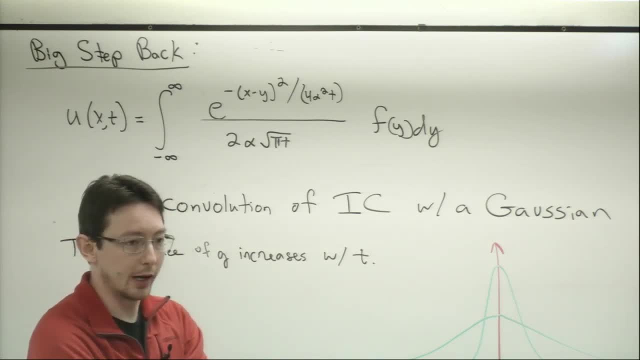 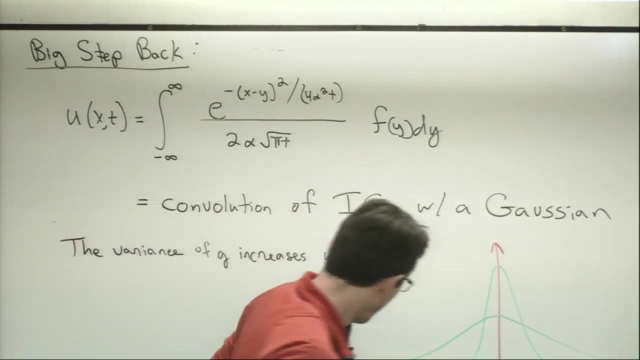 Okay, it's not exactly a time saver. It's like we get a new perspective on the system. Okay, so we get this entirely new perspective by doing the Fourier transform, which is that in the Fourier, so in space, we have space. 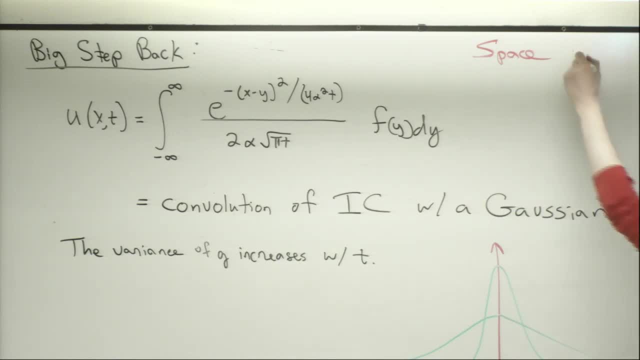 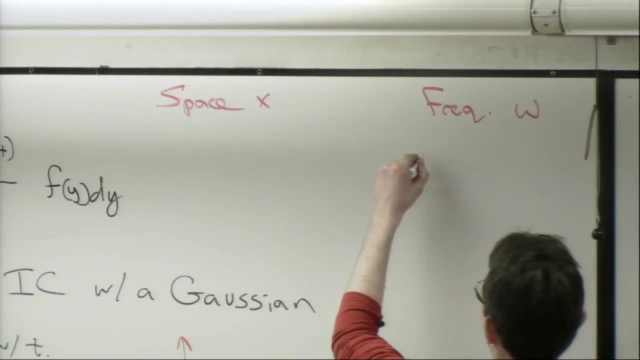 and we have frequency domains. So let's try and understand the Fourier form together. and we have frequency domain, right? So we have x and we have omega And what we saw is that in the frequency domain we had g, hat. u equals g hat times f hat. 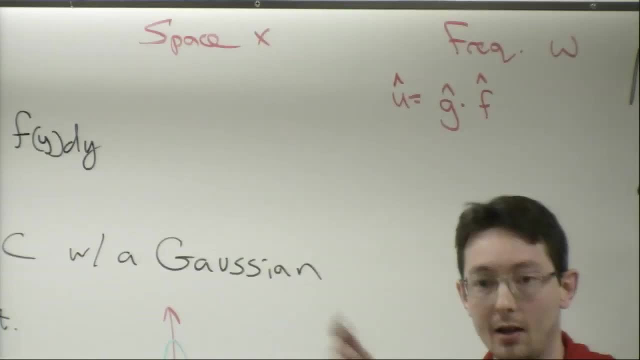 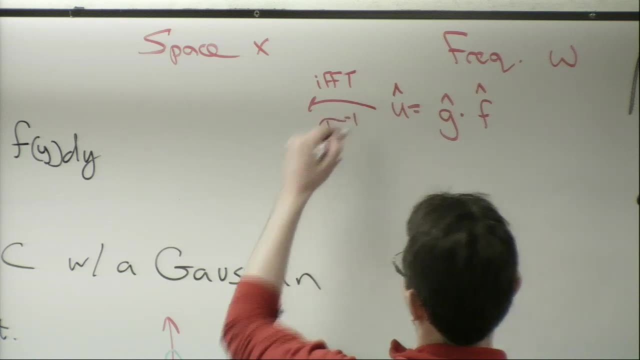 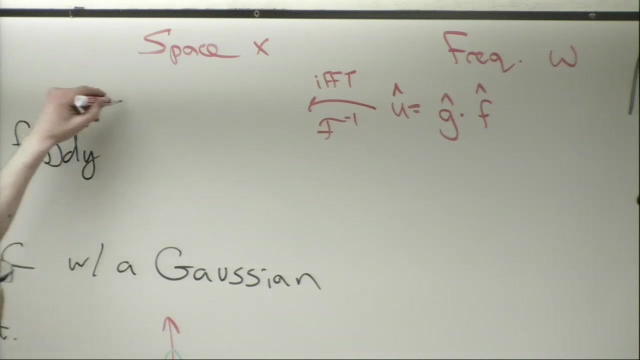 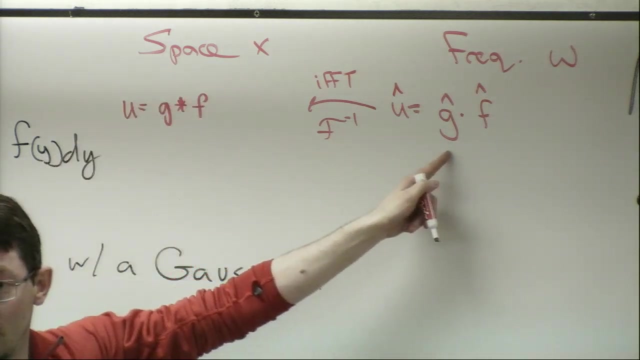 u hat is just the product of my Gaussian times, my initial conditions. But in space, when I fft, when I inverse Fourier transform, this product of two functions becomes a convolution of the functions. So this becomes: u equals g, star f, where g is the inverse Fourier transform of g hat. 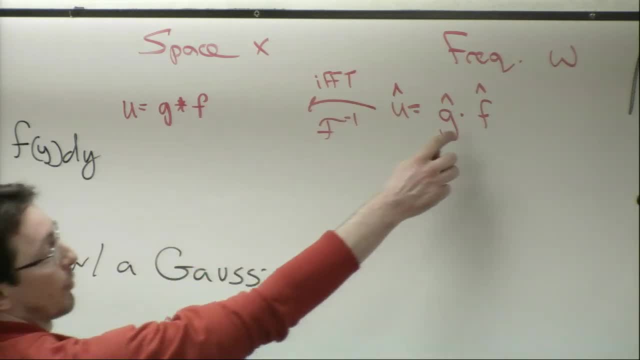 f is the inverse, Fourier transform of f- hat, And now this product becomes a convolution in space. So this is one of the major properties that we find is that it's actually simpler in the frequency domain. The product of this Gaussian was very clear what was happening. 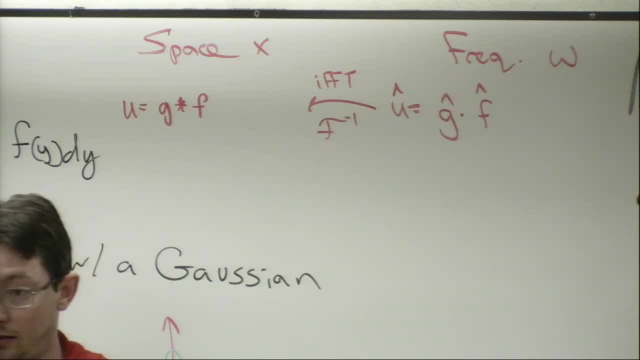 We were damping out every Fourier coefficient at different rates according to this Gaussian decay In space, it's a little less clear. This is what we would get from separation of variables. So I actually like thinking about the system in the frequency domain because it makes a lot more sense. 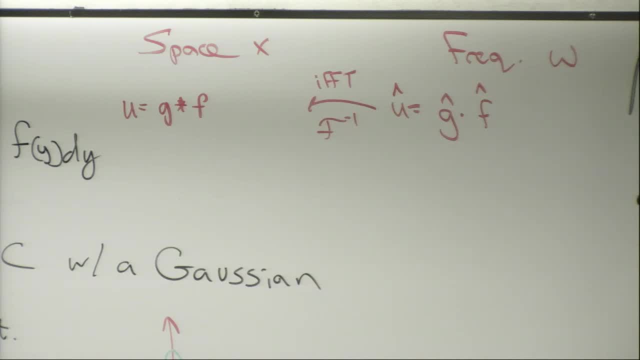 We have damping of all of the frequency components of my initial condition And getting this sentence. you know that the solution is convolution of my initial condition with a Gaussian. we'll find that that's really the benefit of working in the Fourier and the Laplace domain is that we get this very. 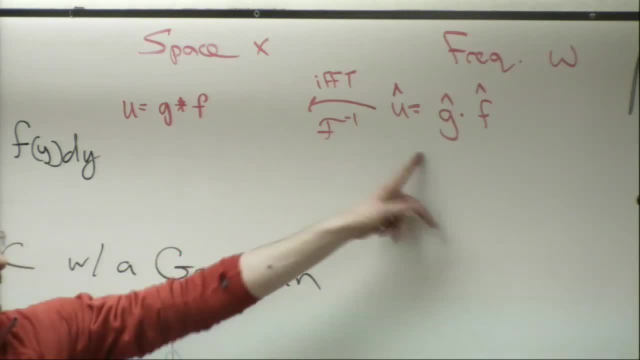 very simple, physical intuition, And that's given by this connection. So I'm going to elaborate more on why this is important on Monday, And we're also going to see that this allows us to do numerical computations. So we're actually going to do computations. 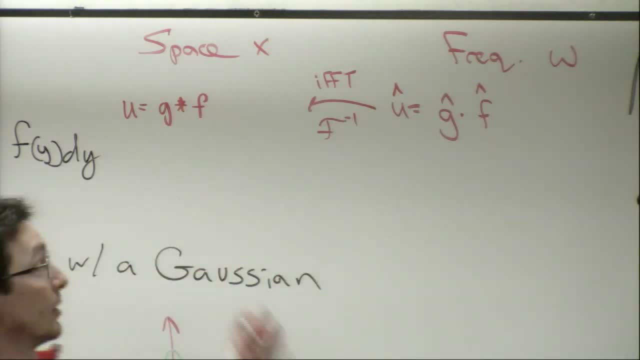 in the frequency domain And everything's going to be much, much simpler than doing computations in the spatial domain. It's more accurate, It's faster, It's easier to code. OK, All right, Thank you.